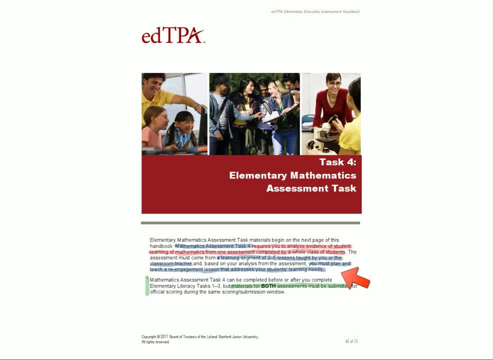 and teach a re-engagement lesson that addresses your students' learning needs. So this is all of it in a nutshell And a simple note down here: Whether you do the literacy tasks first or second, or the math task first or second, all the tasks should be submitted at the same time for scoring, So let's keep that in mind. 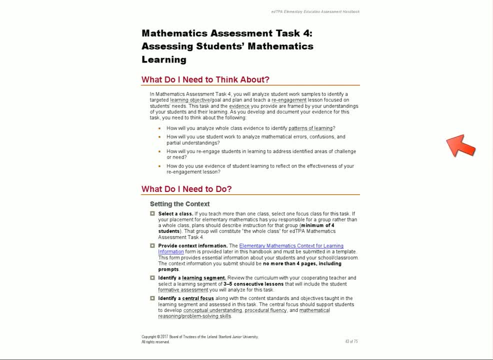 Now, as with the other tasks, there are four sections. The first two are: what do I need to think about and what do I need to do? If we look up here in Mathematics Assessment, Task 4,, you will analyze student work samples to identify the problem or the problem of the. 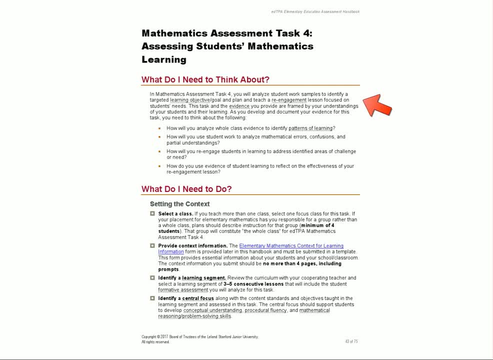 a targeted learning objective and plan and teach a re-engagement lesson focused on students' needs. Students' needs are going to come up throughout this task, so keep that in mind. This task and the evidence you provide are framed by your understandings of your students. 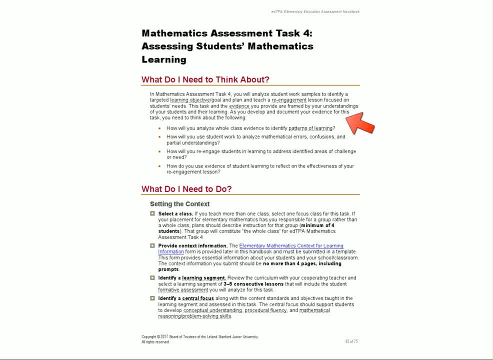 and their learning As you develop and document your evidence. for this task, you need to think about the following. So let's take a look at this bulleted list here. So you will need to think about how you will analyze whole class evidence to identify patterns. 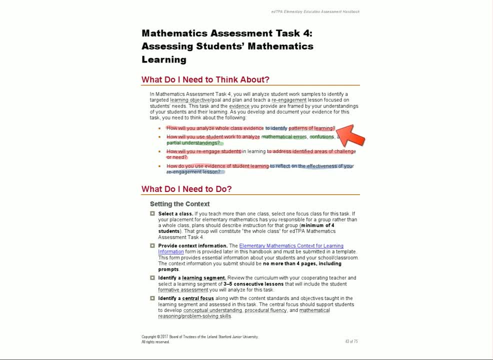 of learning. Patterns of learning is a term, a phrase, a way of thinking about the analysis that you will need to hold on to, and I'll talk about that more in depth in a moment. How will you use students work to analyze mathematical errors, confusions? 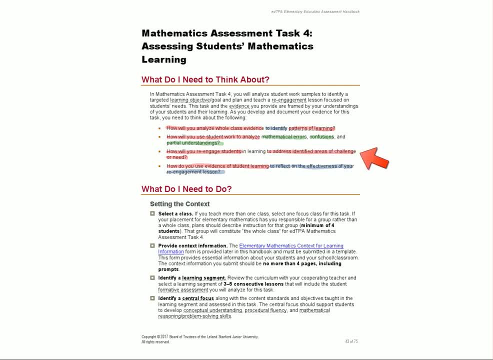 and partial understandings. How will you re-engage students in learning to address identified problems? How will you re-engage students in learning to address identified areas of challenge or need? So, areas of challenge or need, struggles, those things will come up, come up throughout the task. And then how do you use evidence of? 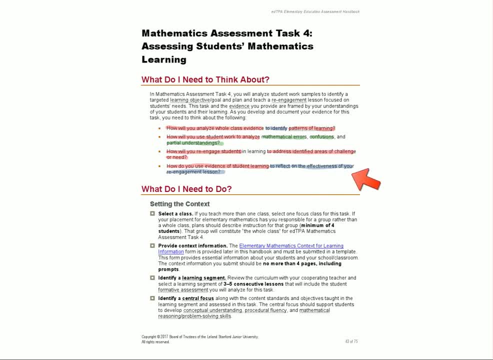 student learning to reflect on the effectiveness of your engagement lesson Alright. that will come up in more detail later as well. Let's think about what I need to do. First off, you will need to select a class And this class, if you 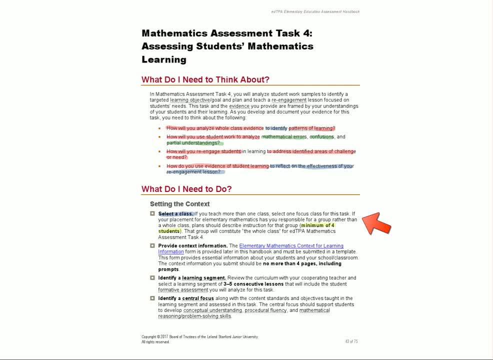 teach more than one class, select one focus class for this task, Alright, And this class needs to have a minimum of four students in this group. So if you're teaching a group of students, there have to be at least four students in that. 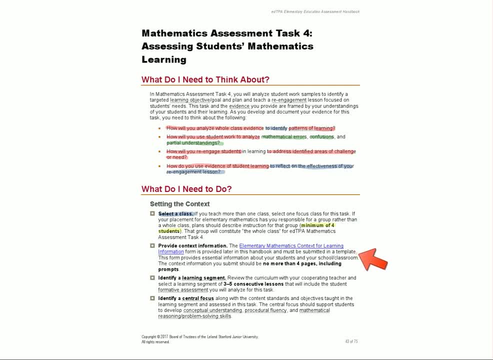 group to consider it a class. Now, something particular to the mathematics task is that you need to have a mathematics context for learning. Now, you did such a thing, or are doing such a thing for the literacy portion, but you need to do similar work for the math task. 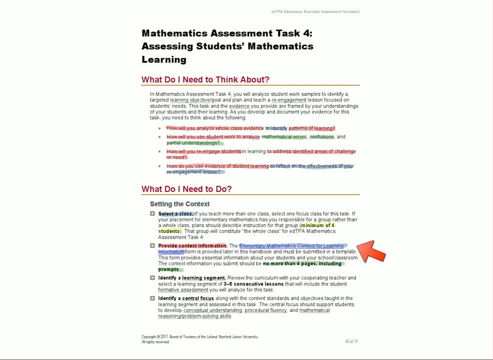 A lot of the things will be similar in terms of students' needs and such, but there will be particular questions about the mathematics program And that helps the evaluator for this assessment know what kind of school you're in, who your kids are, what kinds of things do they bring to their learning? 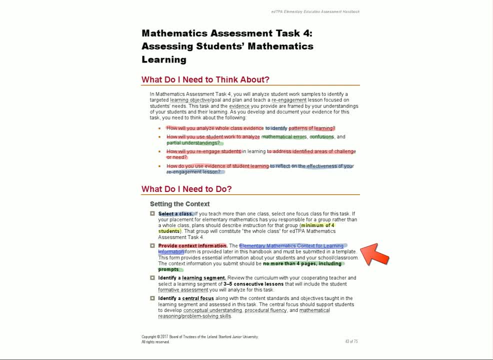 and the shape of the math program, what kinds of text or materials are most frequently used in your program? And this context for learning should be no more than four pages. Next, you will need to identify a learning segment As they suggest. work with your cooperating teacher to find a sequence. 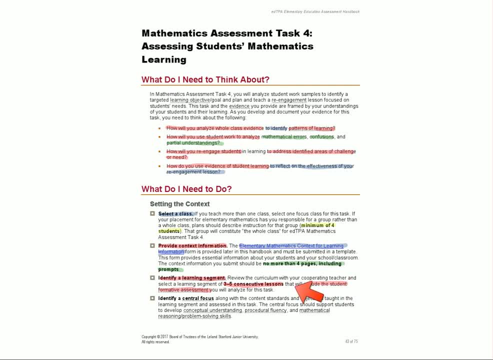 of learning segments: A three to five consecutive lessons segment that will include a student formative assessment that you can analyze Now. I'm going to talk more about this in a moment, but before we get started, you want to think about these three to five consecutive lessons, this learning segment. 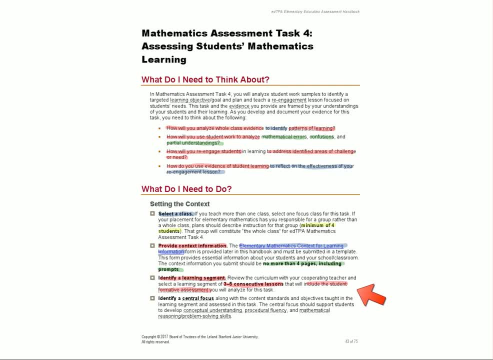 as being rich in mathematics in a number of different ways. It shouldn't be just focused on procedures. It shouldn't just be Some kind of activity that doesn't reach for kids deeper understandings of mathematics. It should also be a sequence of lessons that allows students to show their work in depth. 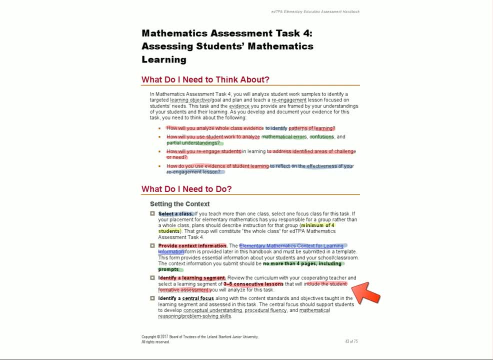 and in multiple ways. All of those things will help you later on when you are doing your analysis of their assessment. So that's going to be something critical to this task is choosing the right set of lessons that set you up to consider conceptual understanding. 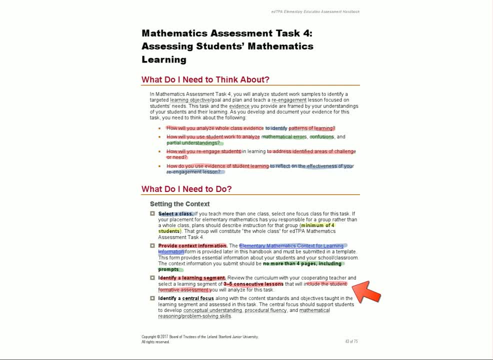 to consider procedural fluency and to consider problem solving and mathematical reasoning. And lastly, on this page, you want to identify a central focus along with the content, standards and objectives, so you need to have both of those things. What is at the heart of this series of sequence of lessons? 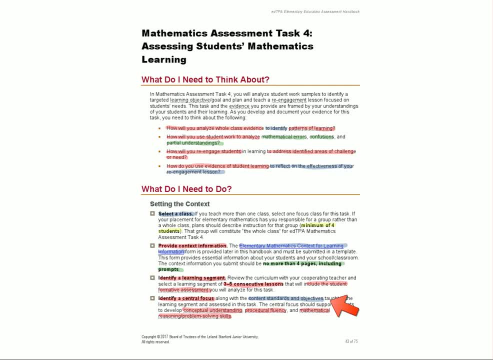 What are the big ideas coming out of this lesson segment, this learning segment of three to five Three to five lessons, and then what content, standards and objectives sit alongside that and make sense? And again, the three things we're going to care about throughout this task: conceptual understanding. 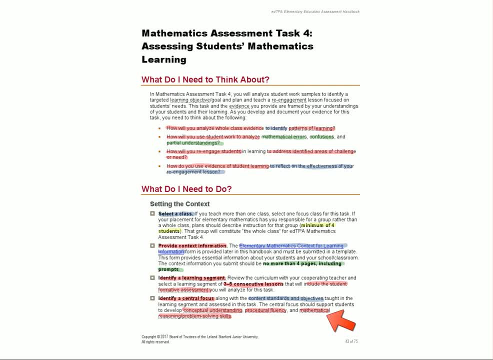 procedural fluency and mathematical reasoning and problem solving skills. All right. So it says the central focus should support students to develop conceptual understanding, procedural fluency, mathematical reasoning and problem solving skills. All right, So these three are the most important part, the biggest consideration throughout this task. 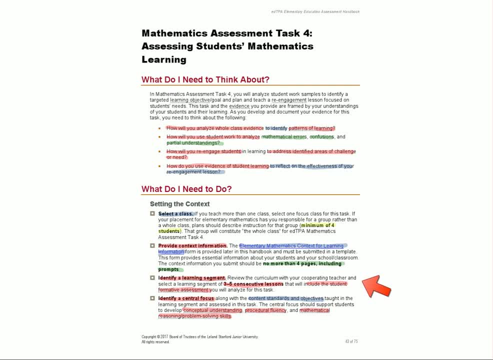 So a couple things to hold onto before we move on. All right, These are the things you'll be doing in this task. You'll be giving a formative assessment. You'll be analyzing students' work on this assessment. Based on that, you're going to design a re-engagement lesson. 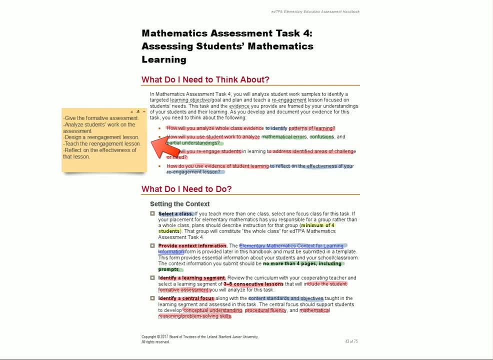 You will teach the students. You're going to teach the re-engagement lesson and then, after you've taught the re-engagement lesson, you're going to reflect on the effectiveness of that lesson. So these are the things that you'll be doing for this task four. 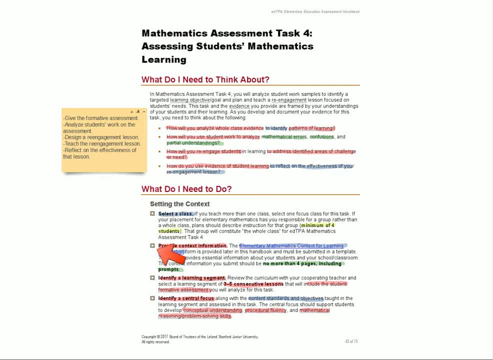 Next, again most important. this is most important. The learning segment should give students opportunities to develop conceptual understanding, procedural fluency, mathematical reasoning and problem solving, And I'm going to be saying those things often throughout this task just because they are that important. 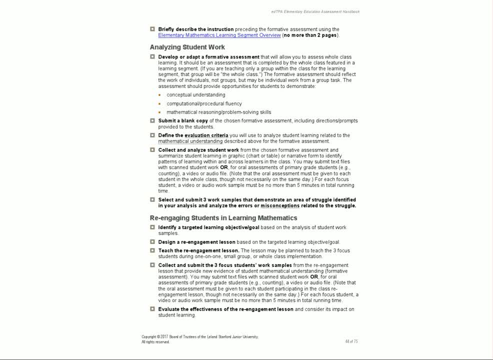 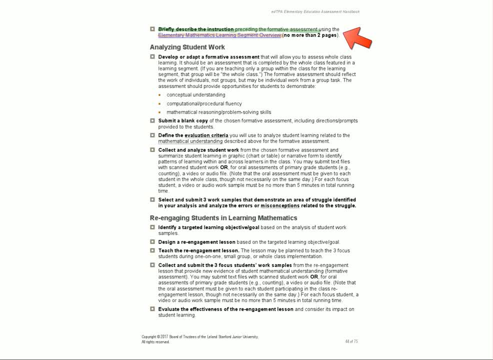 classroom around the mathematics that set up the formative assessment and give some context for what students were doing before the assessment. All right, now this next section is going to be probably the thickest section of the task, so let's go through this step by step. 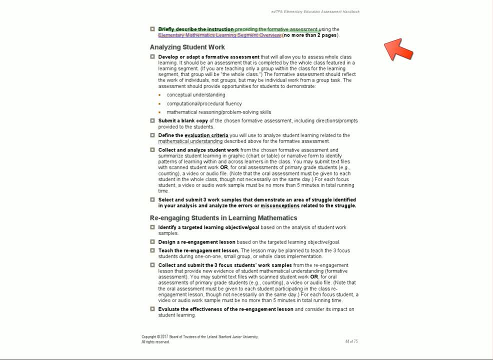 The next thing that you'll be working on is analyzing the students' work. Now, first, you're going to have to develop or adapt a formative assessment. It should be an assessment that is completed by the whole class, and the formative assessment should reflect the work of individuals. All right, 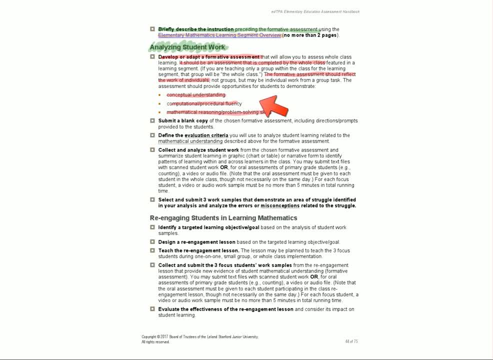 and around these three things: conceptual understanding, computational and procedural fluency, mathematical reasoning and problem-solving skills. Now, the important thing here is that you're going to have to develop or adapt a formative assessment. It should be an assessment that is based on the data that you're collecting. This is what you're going to be. 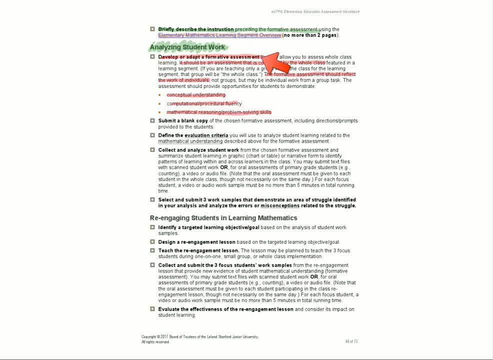 using to develop or adapt a formative assessment. So it's going to be a formative assessment. Now you're going to have to develop or adapt a formative assessment. This is what you're going to be using: to develop or adapt a formative assessment Instead of just using a formative assessment. that. 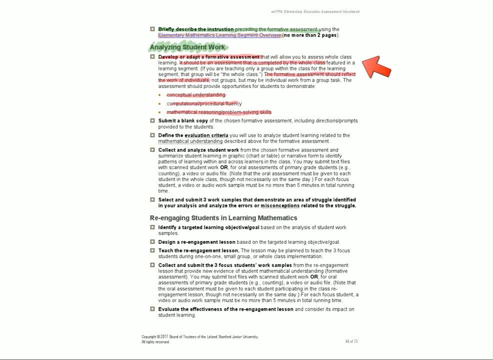 might come out of the given text or the given program. in your classroom you might start with that given assessment and then rewrite it and remake it so that it better sets students up to show these three things. All right, so these three things are always at the top of your consideration. 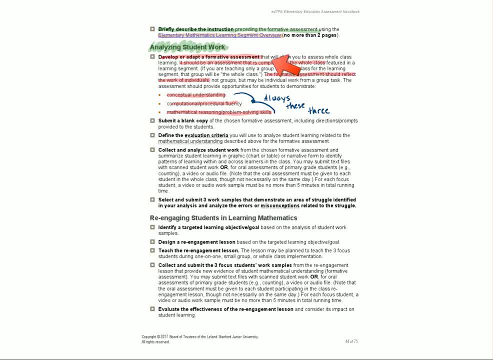 All right. so make sure that your assessment sets you up to be able to see how students are doing or their understandings regarding these three, always these three, Now practical matter. make sure you have a blank copy of the assessment to submit Now. more importantly than that, 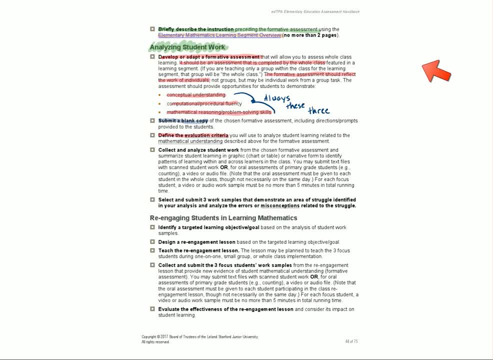 more important than that is you need to define the evaluation criteria And the evaluation criteria. however you set them out, they should hit again these three. All right. so consider your evaluation criteria as looking for some kinds of conceptual understanding, looking for some evidence of procedural fluency, and your criteria? 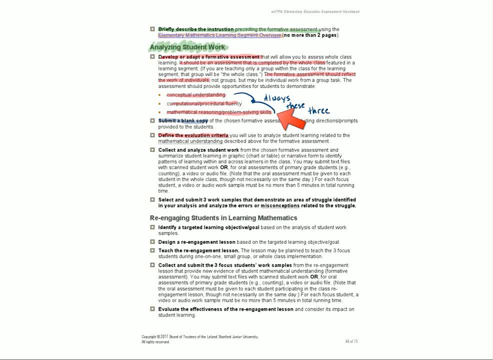 looking at the means and methods students go about their problem solving. So the evaluation criteria, the most important part, or the most important part that you want to make sure you set that out in your formative, for your formative assessment should always go back to these three. 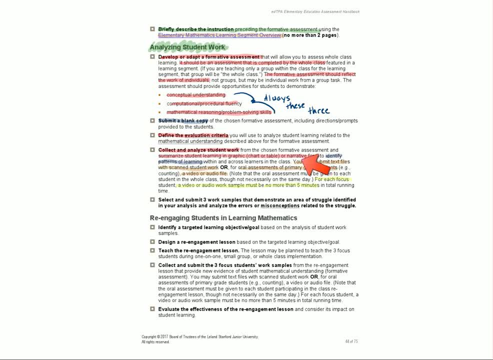 Now the big part here is you're going to be collecting and analyzing the students' work and you want to summarize students' learning from your analysis on some kind of graphic, chart or table. You might choose to do it in narrative form. graphics, charts and tables tend to offer you some opportunities to look for patterns of learning. 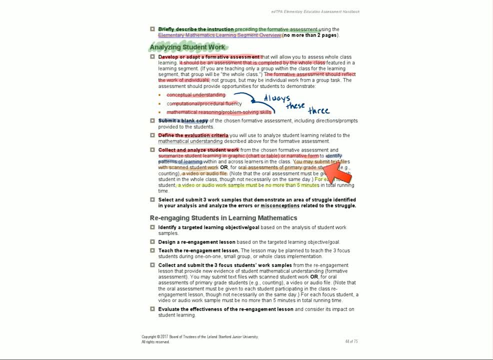 that aren't necessarily as available in the narrative form, and i'll share some of that in a moment. okay, um, so here's some details about how you might go about this. you may submit text files with scan student work or oral assessments for primary grade students. video or audio file will. 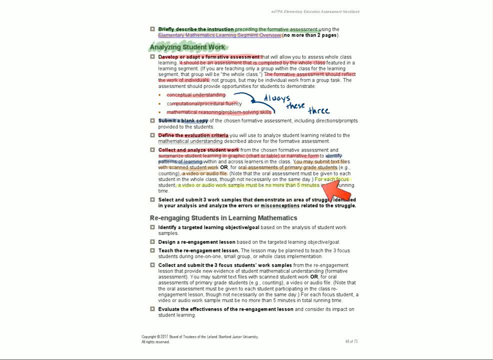 work. all right. for each focus student, a video or audio work sample must be no more than five minutes in total running time. all right, um? so let's go over a couple things here. first off, what are patterns of learning? what's nice here is: ed tpa describes patterns of learning in. 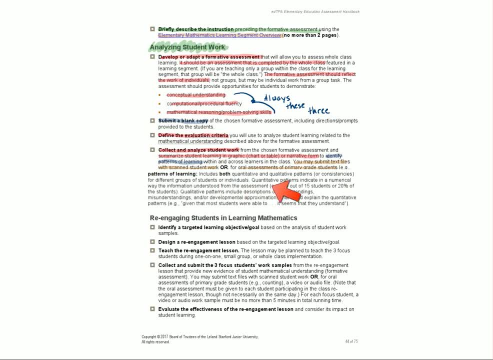 terms of mathematics here. so let's look at this. patterns of learning includes both quantitative and qualitative patterns, or consistencies for different groups of students or individuals. quantitative patterns indicate in a numerical way the information understood from the assessment. for example, 10 out of 15 students or 20 of the students. so when you're 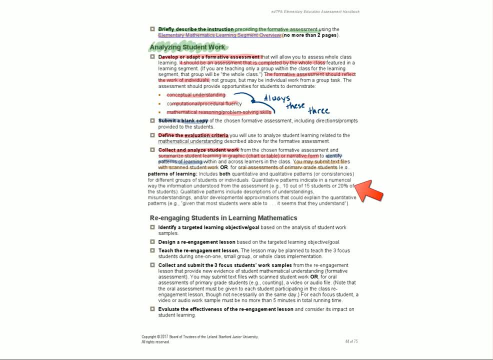 writing this up in your commentary. you might want to use this kind of, this kind of phrasing: three of the 15 students, or eight of the 15 students, or, you know, 19 of the 20 students, and that's a good way to describe things quantitatively in terms of patterns of. 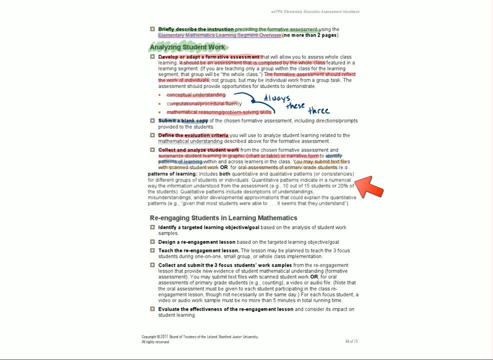 learning. three of the 15 students were able to add, unlike fractions, with and without procedural error. okay, patterns like that. qualitative patterns include descriptions of understandings, misunderstandings or developmental approximations that could explain the quantitative patterns. so, for example, given that most students were able to, it seems that they understand. so keep these in mind when you're writing about patterns. 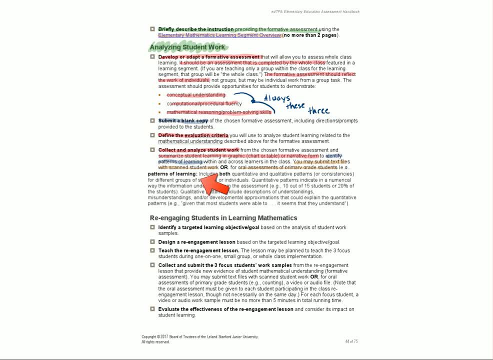 of learning. when you get to the commentary, using the term patterns of learning is probably a good idea. i noticed, or i see within my analysis, these patterns of learning, or this pattern of learning was evident for three of my 15 students, so keep this in mind. now i want to go into more depth. 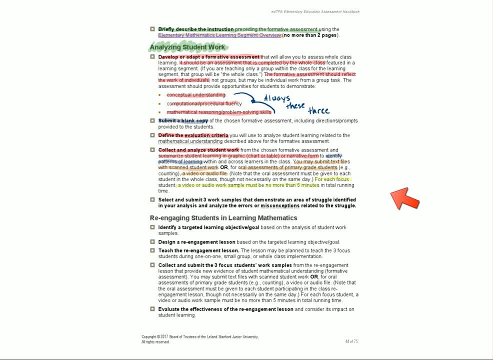 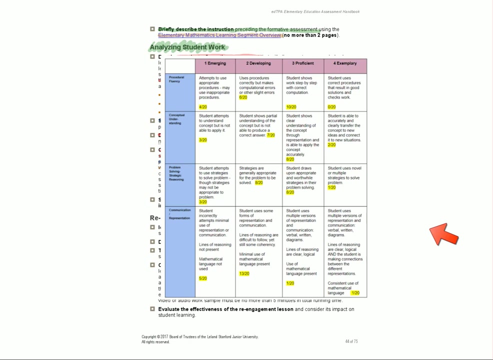 about the chart, all right. so first off, since there's such an emphasis on concepts, computation and problem solving, you should organize yourself around that. so here's an example of criteria that have been set out around those topics. now, if we take a look at this chart, you can see that this particular rubric talks about, or. 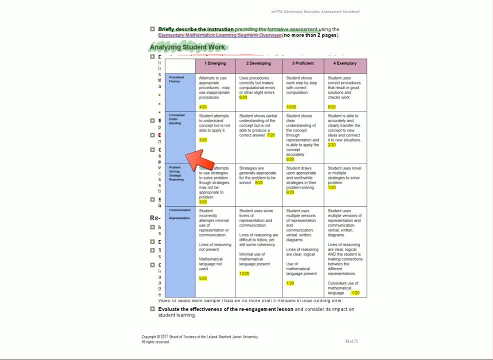 sets out procedural fluency, computational understanding and problem solving strategic reasoning. they also include: this particular rubric talks about procedural fluency, computational understanding and problem-solving strategic reasoning. they also include the suit in the chart, which is these three of the five ways of understanding: behavioral fluency: thicker understanding. this is a walk-through of a concept and features language using the terms of the concept and how to fight. 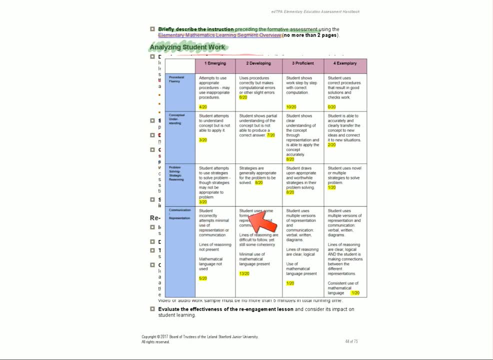 also includes communication representation. So you're not limited to these three, but you must include these three some way. And in this particular rubric you can see that the descriptors set out what levels of understanding might be evident. So if we take procedural fluency, 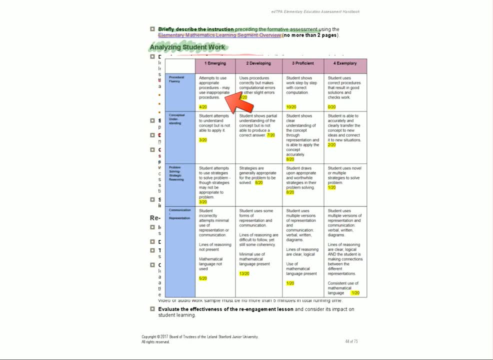 emerging or the lowest level attempts to use appropriate procedures may use inappropriate procedures. The next level up, developing, uses procedures correctly but makes computational errors or other slight errors Proficient. so this will be grade level. Okay, so three is what we're. 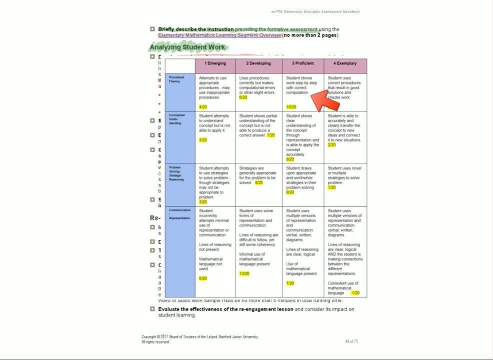 hoping for at least. Student shows work step by step, with correct computation And then exemplary, what might be above and beyond. Student uses correct procedures that result in good solutions and checks work, So something that goes beyond the level of understanding. So, if you're looking, 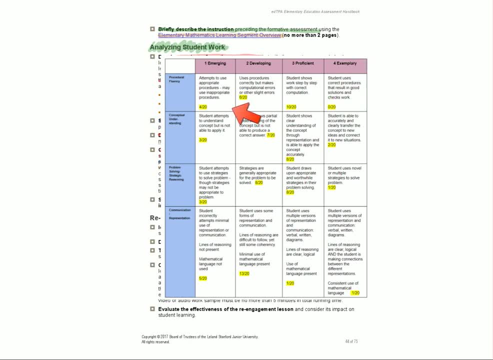 for patterns of learning. you can start looking for patterns of learning. So if we look along here, we can see that there are four of the 20 students who are emerging. So if we look along here, we can see that there are four of the 20 students who are developing. So if we look along here, 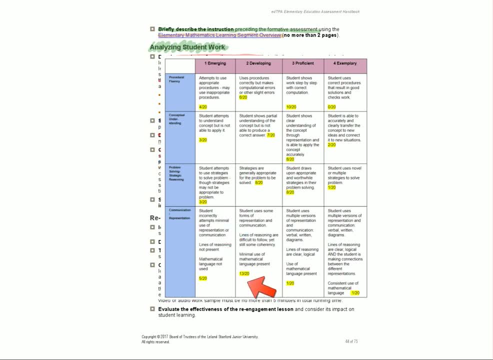 we can see which areas had the greatest struggle. So if we went down here and it was communication representation, you can see that students struggled more. But if we go up here we can see also that in problem solving strategic reasoning we had 11 students of the 20 not meeting proficiency. 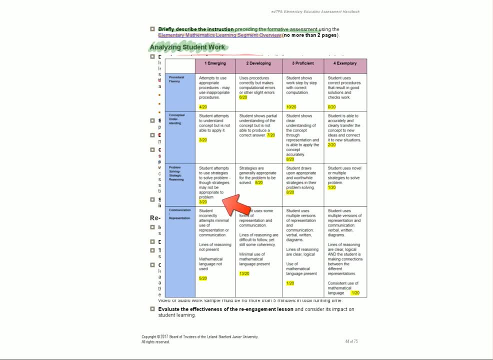 So 11 students And these three students. the student attempts to use strategies to solve problems. Those strategies may not be appropriate for the problem. So if we look along here, these three students struggled in a particular way. So three of my 20 students struggled with. 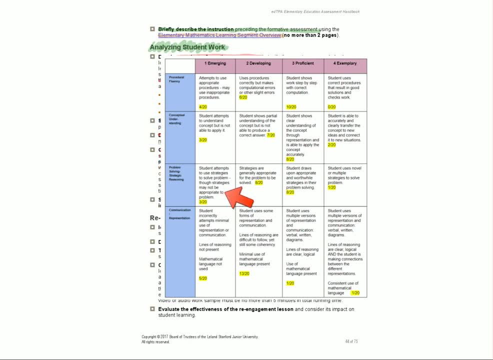 representing the with problem solving, by not being able to show good problem solving strategies or something like that. So this is a pattern of learning. What was up with these three students? All right, And you could imagine for these seven students here what was going on with these seven. 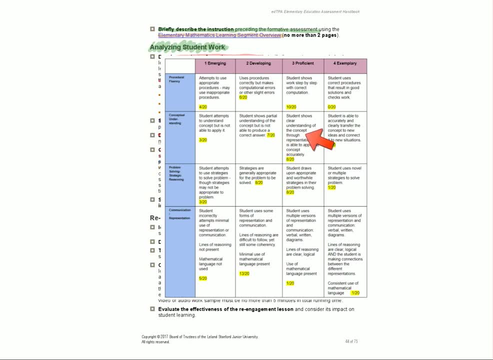 students in regards to conceptual understanding. that kept them from being proficient, And those would be patterns of learning. So if we look along here, we can see that these three students struggled in a particular way. Take a slip of paper here and let me help you with that. Joshua Spring. 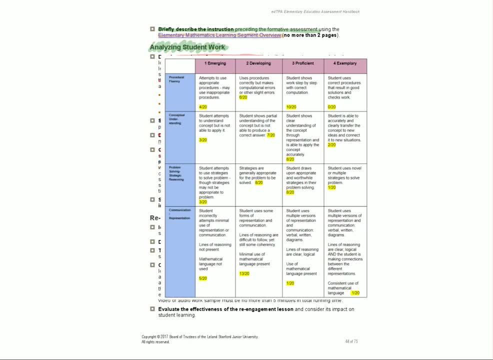 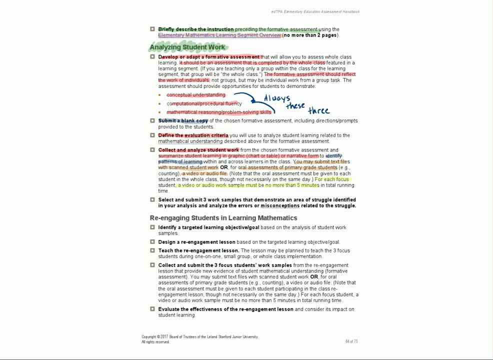 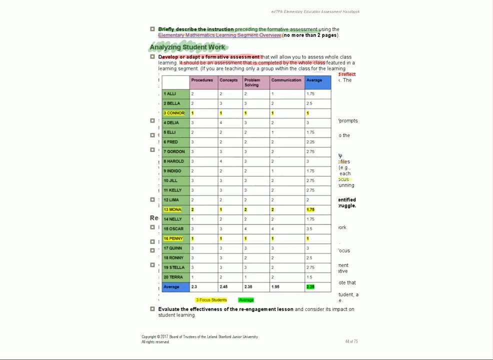 detailed analysis of 16 programs. order of setting and the refraction rules. Joshua Spring serious learning theory assessment and this slide shows us whether students failed or had. Se bizim young student to generate resultsflow and MillerHHHHD Yale's. 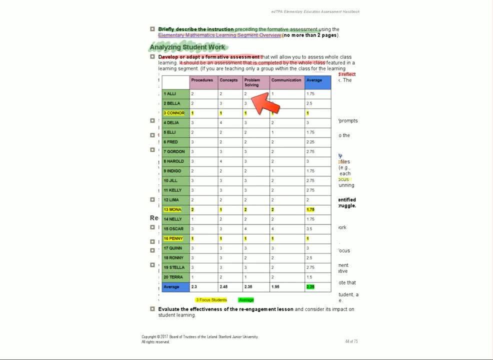 cognitive experience that we could describe in your commentary. So this is one way to look at the charter table. Let's look at a different charter table- that might help as well, And this particular exemplary and these numbers correspond to those different levels. Okay, so a 4. 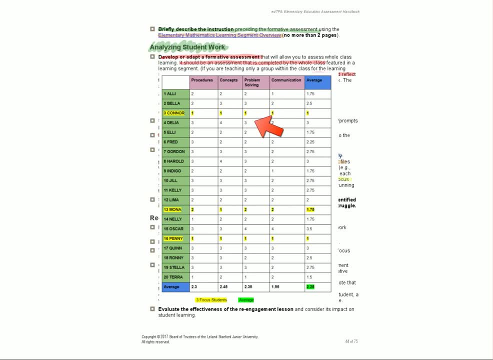 would be a high mark, 4 would be exemplary, 3 would be proficient, 2 would be developing and 1 would be emerging. And from that table you can see that some students are struggling. So here's Connor, who is emerging in every one of 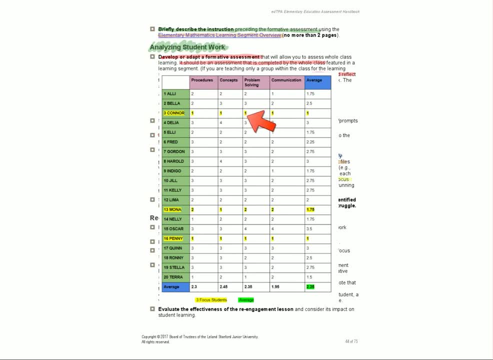 the areas we care about And so, in terms of procedures, concepts and problem solving, the ones that matter for edTBA- this student has great struggles. If we look across, you might see other students like Harold. Harold is doing well, so proficient, exemplary, proficient and lower on. 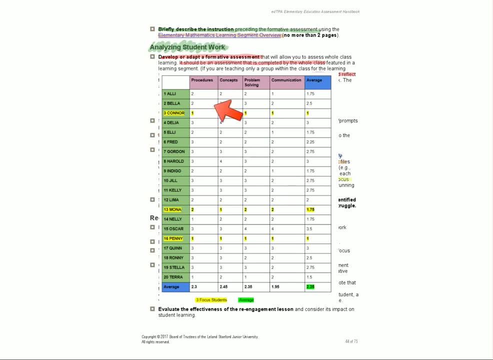 communication. Now, what's nice about this is that looking across this table, we can see how students are doing, but we also can be looking at columns, down the columns, and we can look to see that the students are doing well. So we can see that the students are doing well and we. 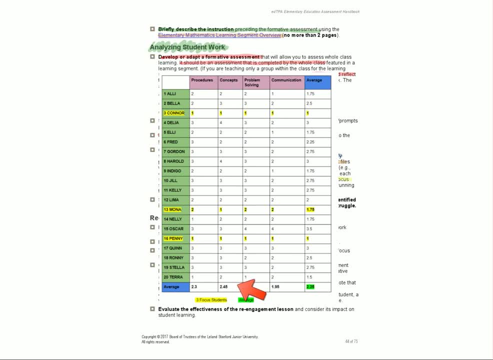 can also look at the numbers. So if we look at the numbers of the understandings or the criteria set out, the communication is the lowest and we could see that conceptual understanding is the strongest. We can also look for bunches or pairs or bundles of numbers to see. you know, what was it with three or four? 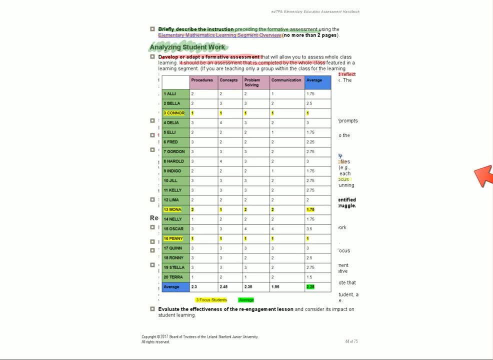 students. What was it with these three students where they were proficient? All of those are good things. We can also look for patterns of learning, So do set yourself up with a good table or chart that gives you good information And, of course, that table, the chart, only works as well as, or as good as, the evaluation. 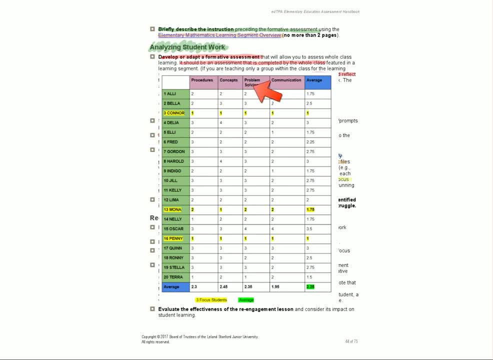 criteria that you've set out. Are you clear about what these are? The other thing to note in this particular chart is that this person has noted who the three focus students are. We'll talk about focus students in a moment. Might as well, start Three. 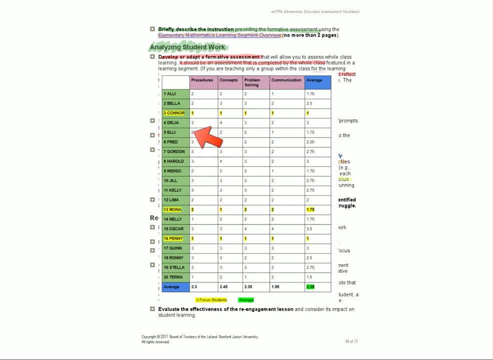 focus students have some particular area of a struggle that should be addressed in the re-engagement lesson. So these three students will be a part of the re-engagement lesson and it could be around concepts. They all were very low in some conceptual understanding of this topic. All right, so that's. 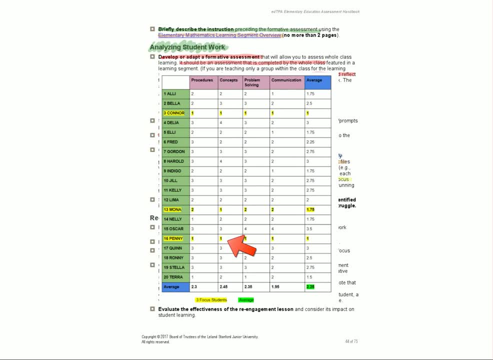 that the significant part of that is that your re-engagement lesson is based on analysis. that comes from a chart like this or from your narrative. Based on your analysis, or based on my analysis, I see that Connor, Mona and Penny are struggling with this particular conceptual piece. 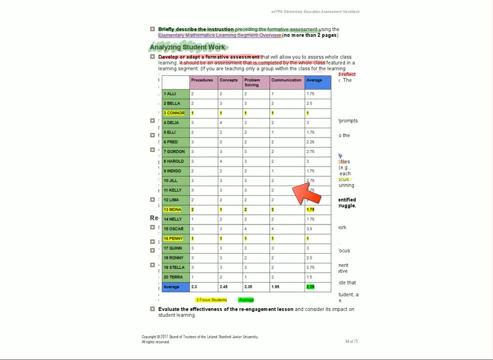 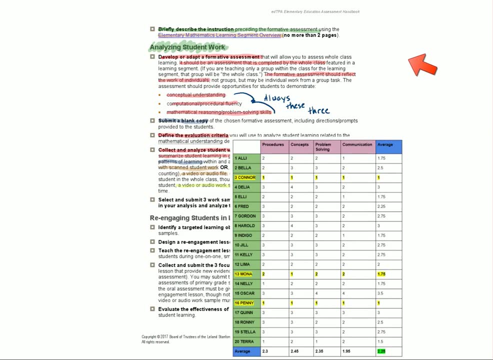 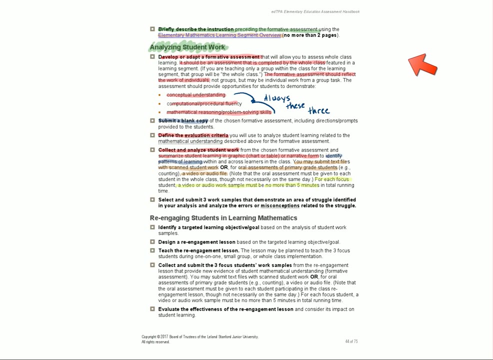 of the mathematics we studied. All right, so everything falls from your analysis of these charts. So let's go on. The next piece is that you want to select and submit three work samples that demonstrate an area of struggle, as we just talked about, about Connor, Mona and Penny. 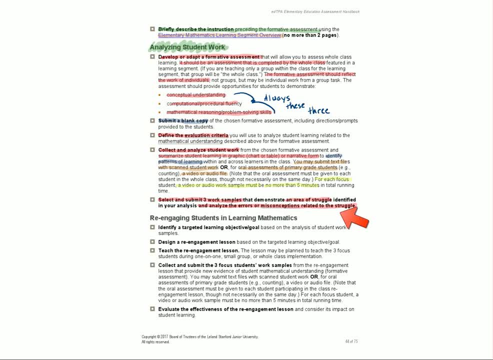 So that area of struggle came from your analysis and you want to analyze errors and misconceptions related to that struggle, And you'll be writing this up in the commentary and I'll get into more detail about that in a moment. So let's go on. 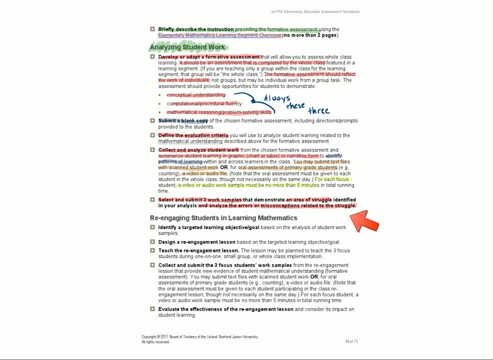 detail in that in a little bit, All right. so that's analyzing student work. This is a significant, important part of task four. All right, everything that you do following that- the re-engaging students to learn mathematics- has to come from your good analysis. 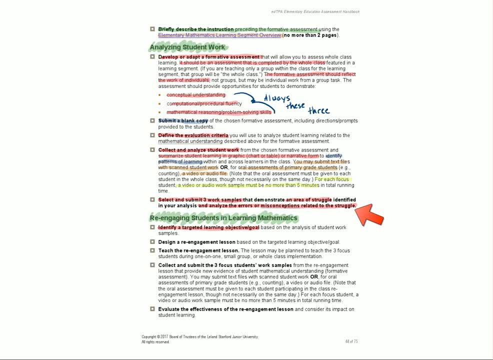 All right. so let's think about re-engaging students in learning mathematics. You want to identify a targeted learning objective or goal, and the important part here is based on the analysis of student work, just as we did a moment ago. Following that targeted 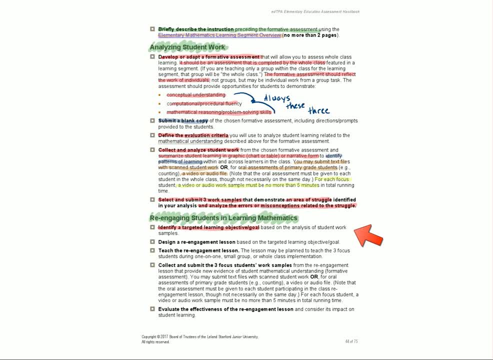 learning objective. where did they struggle? What was the thing that was hanging them up? You want to design a re-engagement lesson? Okay, and it needs to be based on that targeted learning goal. Following that, you will be teaching the re-engagement lesson, All right. 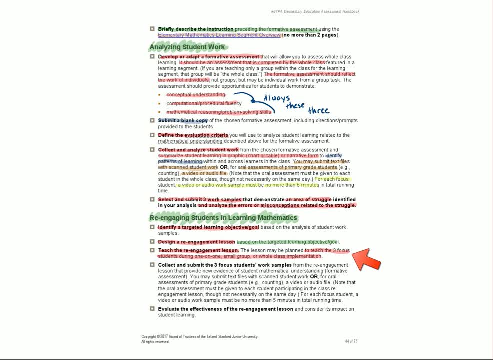 and that lesson needs to be based on the analysis of student work. So let's go on. It needs to have the three focus students in that lesson, but it doesn't mean that they're in a group of their own. In fact, you should have more students in that group. 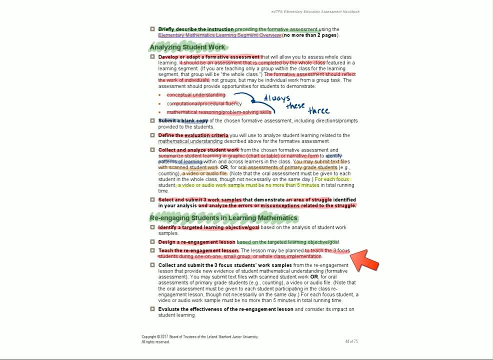 but the three students must be included in that group. Next, you want to collect and submit the three focus students' work samples from the re-engagement lesson and you want to use what work they did from that re-engagement lesson And then you want to use that work sample to talk about to describe their understandings. 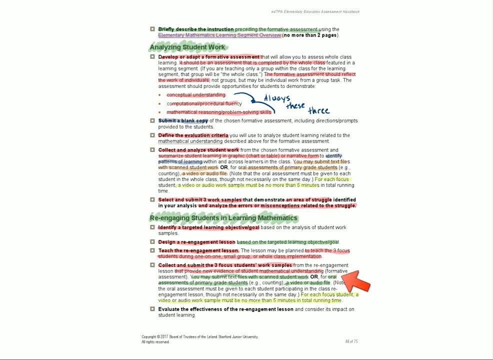 okay To provide new evidence of students' mathematical understanding. and then there's a description of how you might submit this work. If you add audio or video for that work, remember, for each focus, student video or audio work sample must be no more than five minutes in. 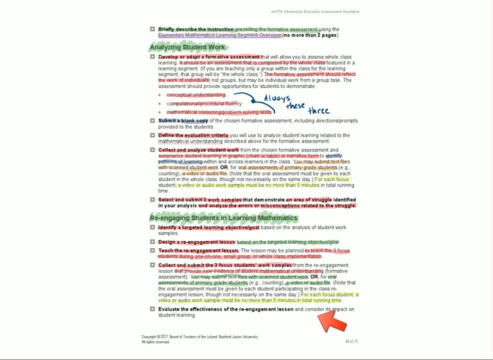 total running time. And then- importantly- this is one of the essential things for this task- you want to evaluate the work sample. So you want to use what work sample you have in the work sample, the effectiveness of that re-engagement lesson and consider its impact on. 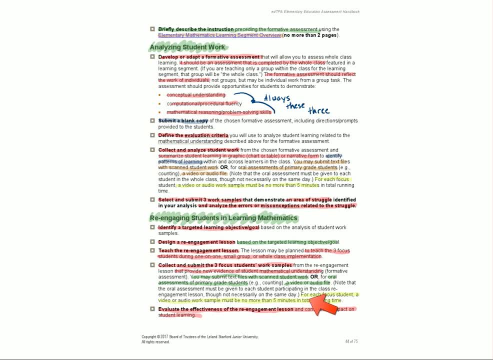 student learning. So let's go over some important things from this particular page- and I'm going to circle back as I've done before. You do need to keep in mind the three as you build your assessment. So, as you develop and adapt a formative assessment, keep in mind conceptual understanding, computational. 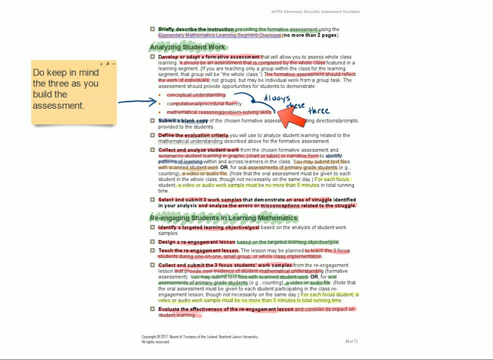 procedural fluency, mathematical reasoning and problem-solving skills- Always these three. When you develop your evaluation criteria- guess what? That's the same thing. Develop your evaluation criteria that will help you to analyze student learning. Make sure that your evaluation criteria address these three. 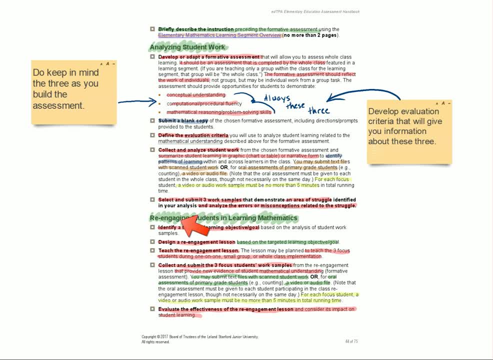 again in some form. Now, when we get to designing your re-engagement lesson, you want to start with the idea. you might even use the phrase based on my analysis, Based on your analysis from the chart or graph or narrative, you were looking for patterns. 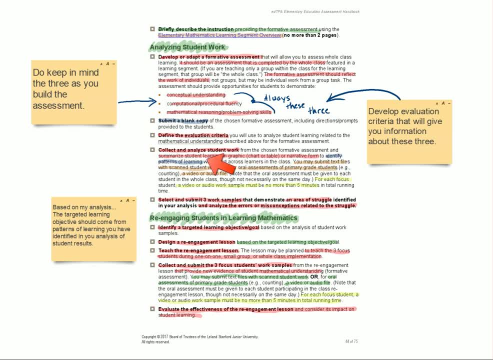 of learning And from the patterns of learning that you've seen, you want to identify or set out a targeted learning objective. The targeted learning objective should come from patterns of learning you have identified in your analysis of the student's results, So keep that in mind. 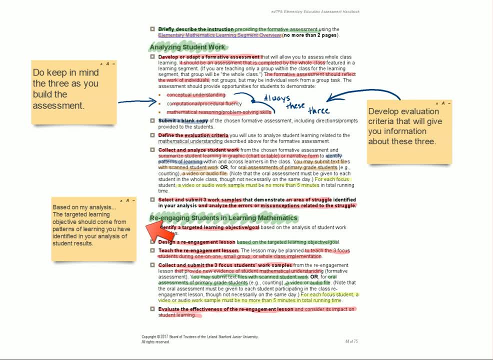 Everything should hold together. And then, lastly, on this page, your analysis should focus on change. This is going to be an important word. Your analysis should focus on change in students understanding of the mathematics. you'll need to need evidence to show this change right. So when you're 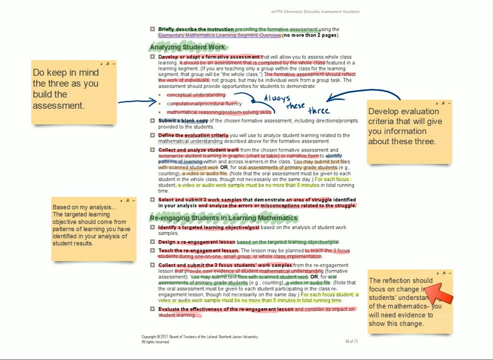 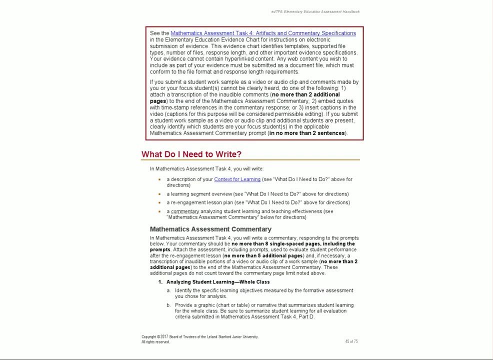 evaluating the effectiveness of your re-engagement lesson. think about: how are my students different? What was the change in their mathematical understanding and how do I support it with evidence? All right now. there's some features that you need to pay attention to in this, So. 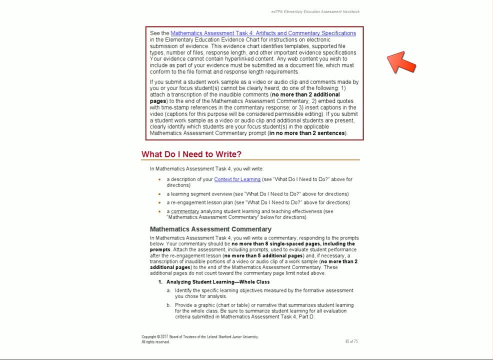 you're collecting lots of information. You're collecting lots of information. You're different kinds of evidence. So the suggestion from edTPA is you look at this section and there'll be a link in your electronic document. See the mathematics assessment test for artifacts and commentary specifications to make sure you have everything in order. 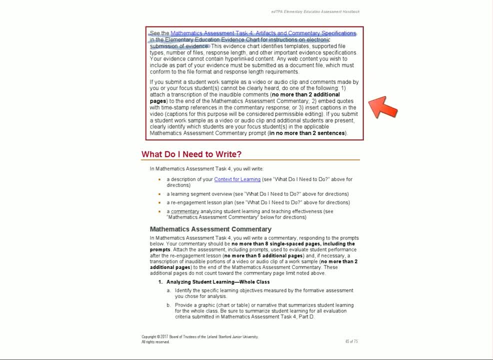 Okay, and then next- and this follows from falls for all the tasks you do. if you're having trouble with audio within an audio clip or a video clip, find a way to support it. Okay, you can add a transcript transcription, you can embed quotes or you can insert captions in the video. Remember, 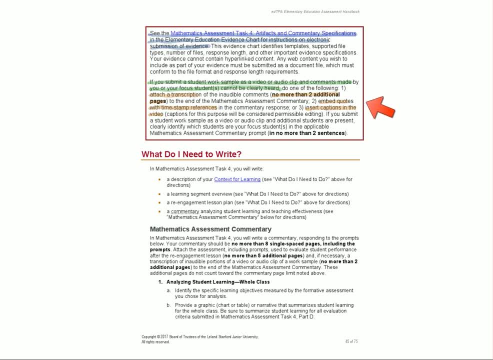 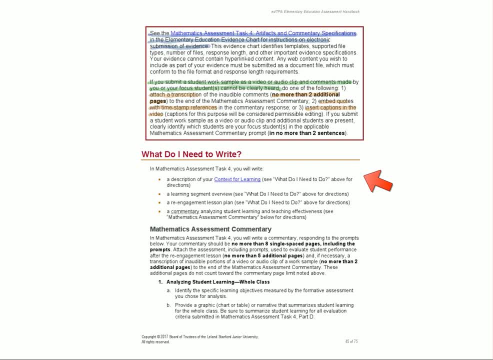 Let's get to the next section. What do I need to write? So, in mathematics assessment, task four, you will write these four things as four pieces: a description of your context for learning. So this is the mathematics context for learning, in which you'll share the program and the materials, as well as who your students are. 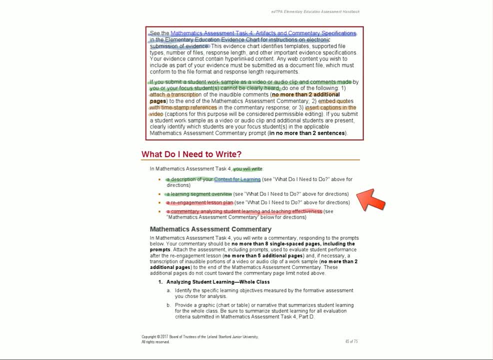 a learning segment overview, because you haven't set out lesson plans for this particular task. You need to say what was going on within those lessons. a re-engagement lesson plan? Okay, And we'll talk in detail about that in a moment- And then the commentary that goes. that fits with all. 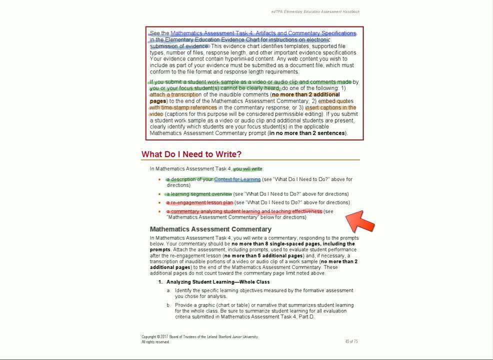 the things that have been mentioned already for this particular task. So let's go ahead and go to the commentary And remember commentary is one of the places where you give evidence of your own good teaching and student learning. So you want to address every prompt in 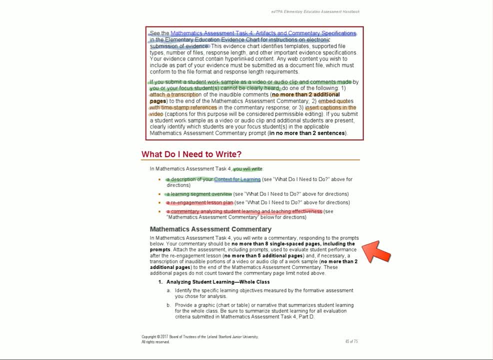 in completely, in full, and address all parts of every prompt and the other piece throughout all the assessment tasks, or all the tasks that you do give lots of good evidence, okay. so let's start with this. this commentary should not be more than eight pages, okay, but you may include these. 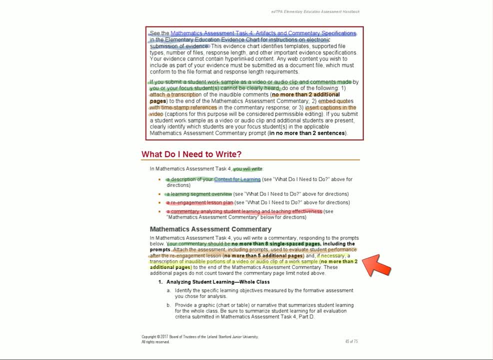 additional things. the assessment itself and, if necessary, transcription of inaudible portions of a video audio clip or of a work sample can be included. no more than two additional pages. so here are your page limitations, so let's get started on what you're actually writing. so analyzing student learning whole class. 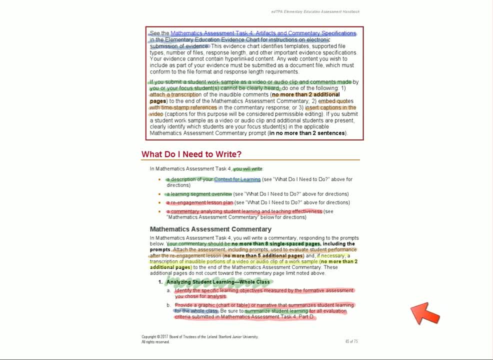 and i want to note something here so you can keep yourself in order. here there are: there's a and b here under analyzing student learning, there's also a, c on the next page so you might flip ahead so you see all three parts of those. so let's get started on this. analyzing student learning: whole class. identify the specific. 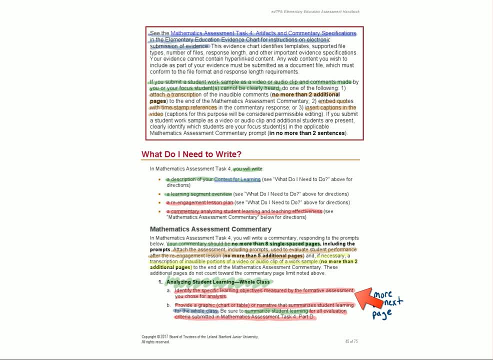 learning objectives measured by the formative assessment you chose for your analysis. okay, so set those out. you might support those and i've seen them supported with um, with content standards, but the learning objectives should be students are intended, the learning segment intended to teach these things to the students in terms of mathematics. the next piece which we've shared: 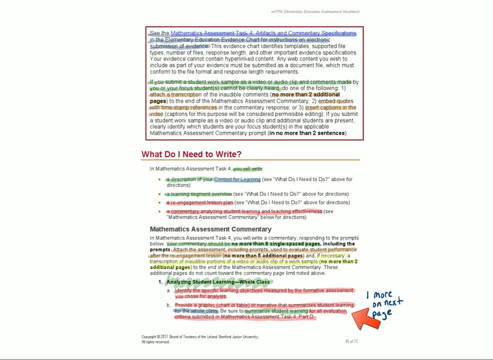 already provide a graphic charter table or narrative that summarizes student learning for the whole class. be sure to summarize student learning for all evaluation criteria submitted in mathematics assessment task for part d. so there's, this is loaded. let's take this apart. you have a choice between sharing a graphic table or chart, so a charter table kind of. 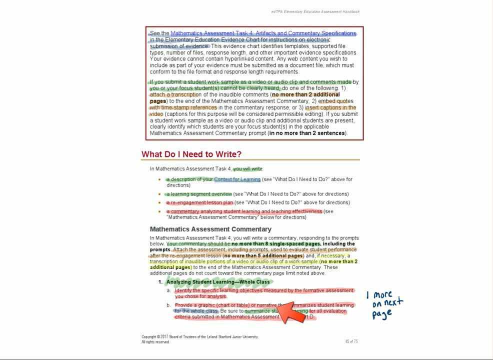 graphic. so that's one choice. or you can write a narrative- all right. so you make a choice between those. but you want that narrative or that graphic to summarize student learning for the whole class, okay, so you need to give whole class results and that summary for student learning should. 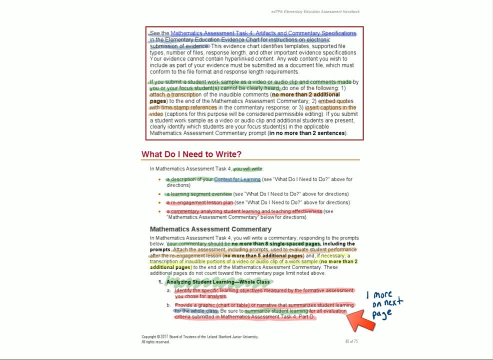 capture or display your evaluation criteria. so your evaluation criteria should be evident in that chart table or narrative. okay, so let's think about the big ideas from this page. first off, on the what do i need to write piece, there are four pieces. let's go through the four. 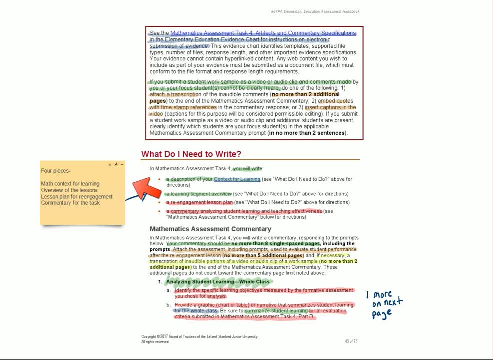 pieces. the first piece is the mathematics context for learning, the second being an overview of the lessons that were taught. that set up the assessment. you need to write a lesson plan for the engagement lesson and then you need to write a commentary for the whole task, which covers all of these other things. 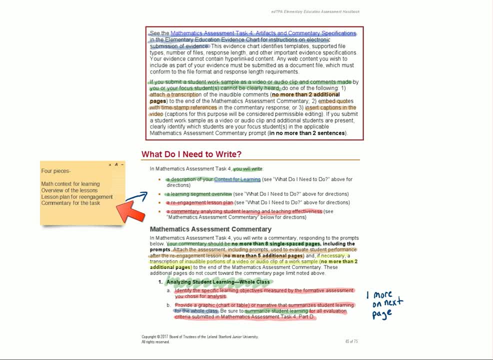 as well, especially the your analysis, and then your re-engagement lesson and teaching. okay, one other thing. um, remember this complicated prompt. here you want to set out your learning objectives- okay, so that's a here: what were your learning objectives? and you want to represent student learning through a charter narrative based on the evaluation criteria. this is the second piece now. 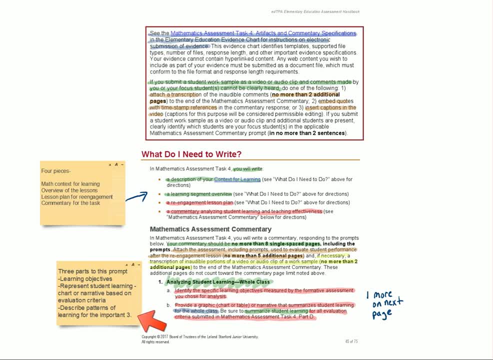 the one that's on the next page is going to be asking you to think about, write about patterns of learning. all right, for the important three. and the important three are conceptual understanding, procedural fluency and mathematical reasoning and problem solving. all right, so let's get to that. 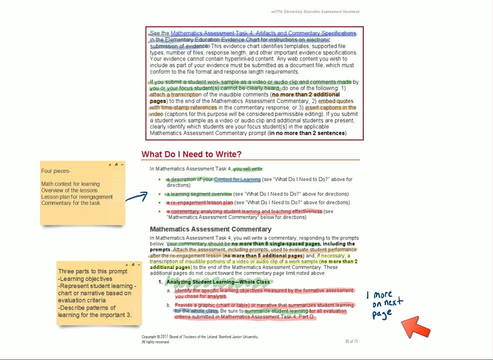 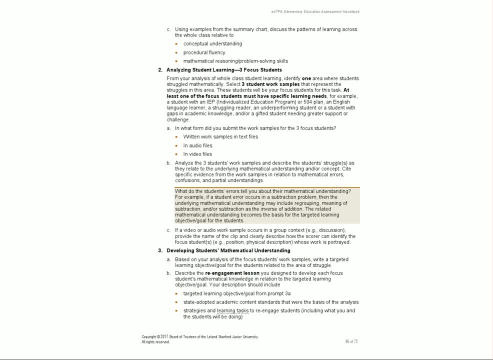 one that's left over on the next page. so see on this page. so, using examples from the summary chart, discuss the patterns of learning across the whole class. okay, two relative two and of course all three are three friends for the math task and, as i've shared with you already, patterns of learning. 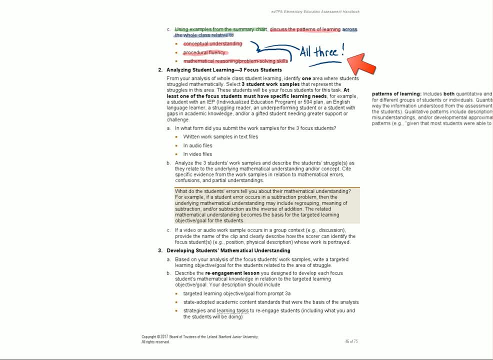 make sure we can see this properly. so the patterns of learning being a little finicky here, all right. so patterns of learning. we can see that the patterns of learning include both quantitative and qualitative patterns, or inconsistent or consistencies for different groups or individuals. patterns indicate in a numerical way the information understood. 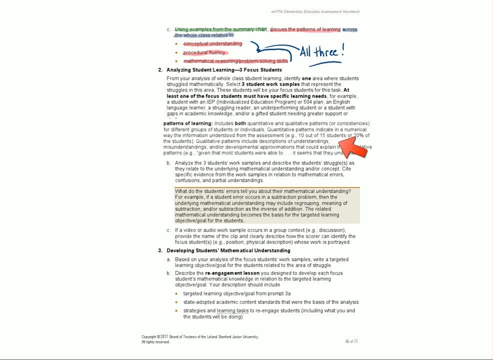 from the assessment examples given: 10 out of 15 students, or 20 percent of the students. okay. so my suggestion for in your write-up for this particular prompt is that you use that kind of phrasing: okay, so, three out of my 15 students, or eight out of my 15? 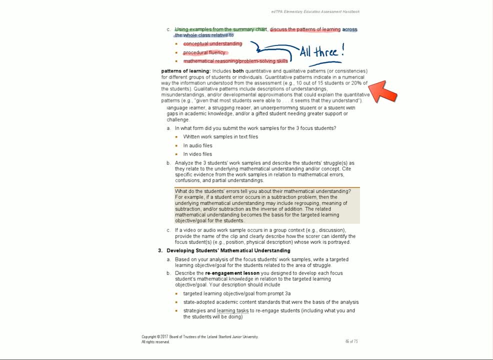 students show this form of conceptual understanding or this misunderstanding. five out of my 15 students did well on procedural fluency, but six of my 15 students struggled with this particular piece of the procedure. so think about everything in terms of patterns of learning. okay, next, oops, let's not do that. 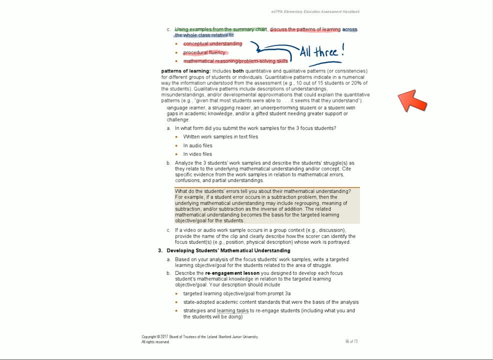 i'll get this straight, okay. the next thing we care about: um, yeah, just give me a moment please. i'm almost there, okay, so let's look at number two. now let's put our patterns of learning aside. patterns of learning have been very difficult for me this morning. 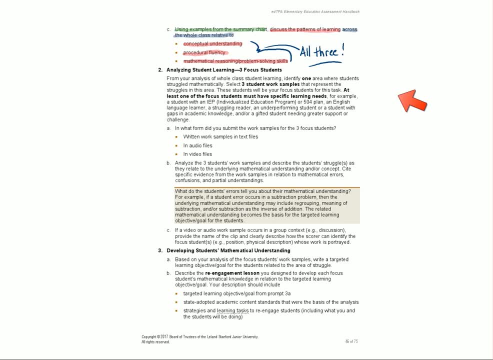 but hopefully they won't be for you. so goodbye, patterns of learning, let's look at number two here. number two: analyzing student learning. we want to think about the three focus students. okay, so essential here from your analysis of the whole class student learning. okay, so you choose your three students. 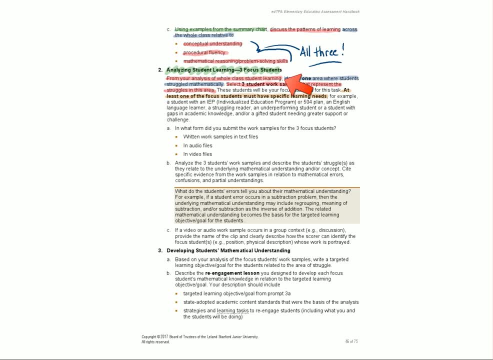 based on your analysis set out in those in that chart or that narrative that you've done for a different prompt. okay, so you want to identify one area where students struggled mathematically. that will become your focus for everything that follows. all right, so you're starting from your analysis of your teaching from the students. work on the assessment. 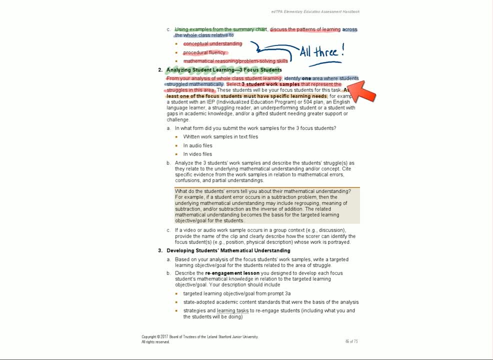 then you choose an area where students struggled and you choose three students to represent that struggle. now, that struggle could be across many students, but you want three students to be focused on in your work, to follow all right, and the suggestion is: at least one of the students. 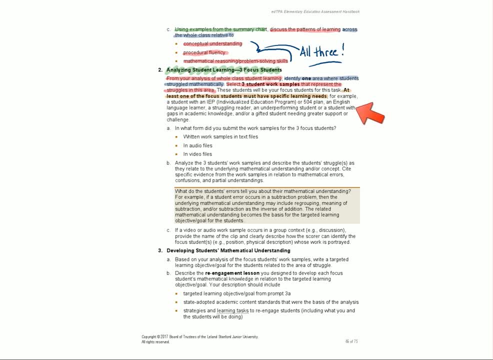 should have a specific learning need and here's some examples here. okay, and when you write up this part later on, when you talk about your three students, you should say what that particular name learning need was. okay, so let's continue. part a: the first prompt is probably the easiest prompt for the commentary in the mathematics. 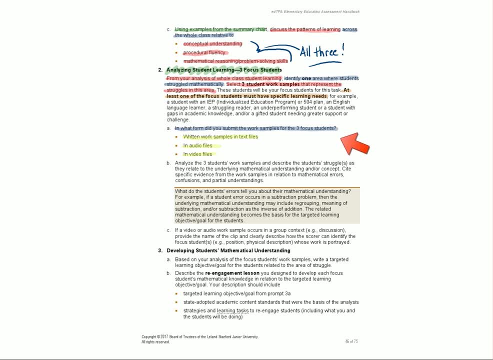 assessment task. what form did you submit work samples for the three students? if they're turning in a paper form, then you write about it. you say it's a text file. if you have an audio file or a video file of their work, then you'll say: that's what i'm working from. okay, let's go to the analysis. 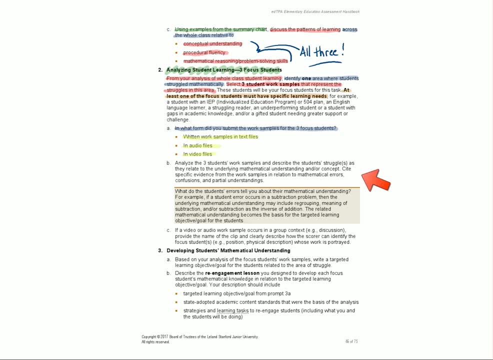 part now. B: you want to analyze the three students work samples and you want to describe the students struggles. okay, so you think about it. struggles needs, struggles. what was it? they are working through and haven't quite gotten yet. okay, based on your analysis of their assessment from the beginning of this, 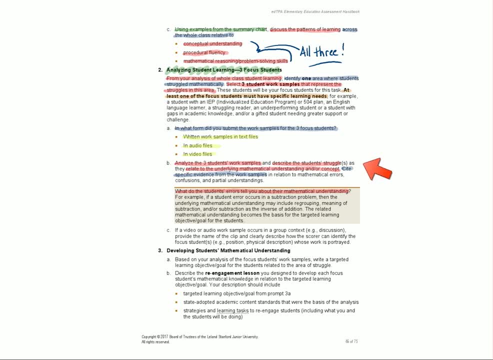 task. what is it they're still struggling with all right now? particularly important here is you need to cite evidence from the work samples about that struggle, so you want to actually write up the problems that they struggled with and then describe what was going on in those problems. that sets. 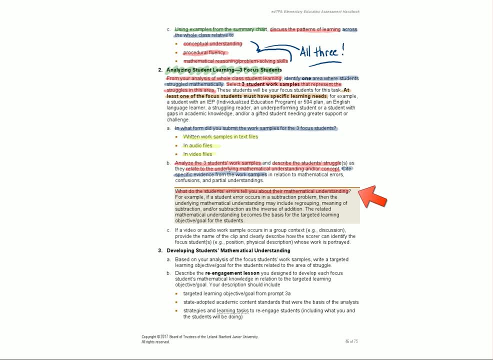 out their struggle okay. and then you can see here what do the students errors tell you about their mathematical understanding, and you can read this example for yourself. all right now. a practical one is C here. if a video or audio work sample occurs in a group context, make sure you identify for the score for the reader of this. 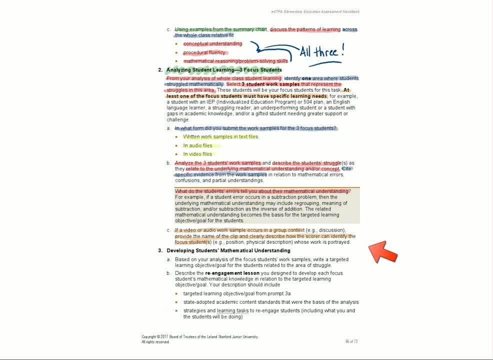 assessment who's who all right now, after you've done this analysis. okay, so you've done your analysis of your three focus students here. you need to set out a lesson and the lesson needs to be organized in a particular way. the first thing that you'll need to do is set out a targeted 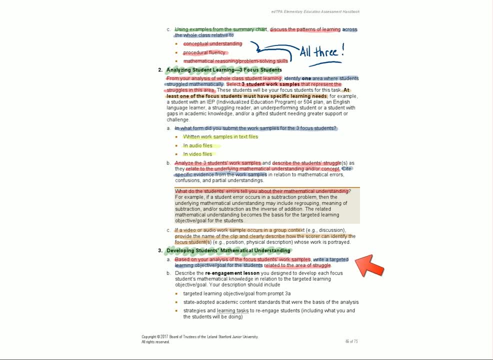 learning objective or goal. okay, and that would. I would suggest using that phrase or that term in your write-up. my targeted learning objective is- and you can imagine what would follow- the other part of this that matters is: you want to, Your analysis, you want to be. you want this targeted learning objective to be based on your analysis of your students work samples. 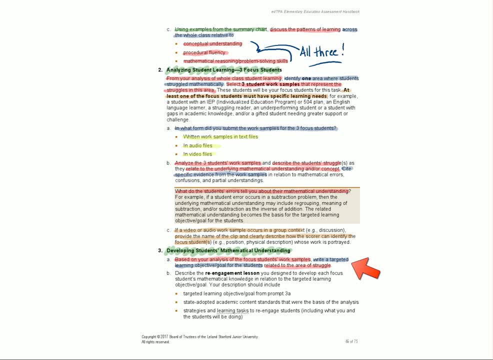 So way to think about this would be based on my analysis of my students work. My targeted learning goal objective based on their struggle will be okay. You can see how all of that fits with this first prompt. right, You're not setting out a lesson about anything. your lesson has to follow from a particular struggle or need. 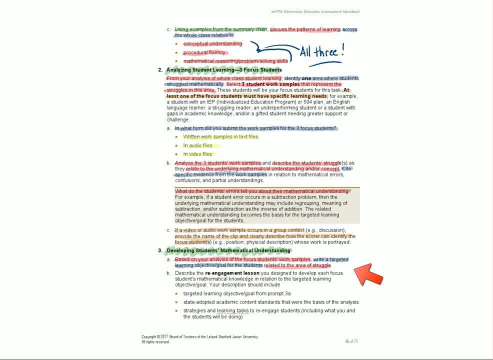 Okay, Now B has five parts and they're broken across two pages. But you want to make sure that you would hit all five parts in your lesson plan, So B is the lesson planning. So we take a look here. Okay, describe the re-engagement lesson. you designed to develop each focus students mathematical knowledge in 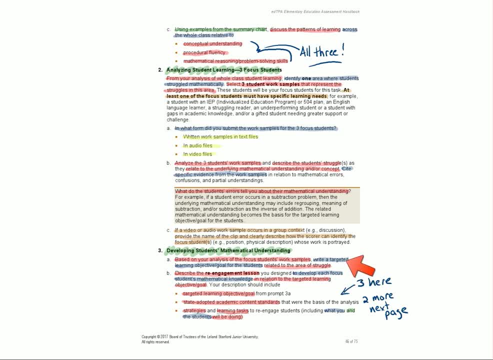 relation to the targeted learning objective or goal. okay, so lesson plan follows from your targeted learning objective or goal and Here are the things that need to be included. The first three, and there are two more on the next page. the first three you need to restate. 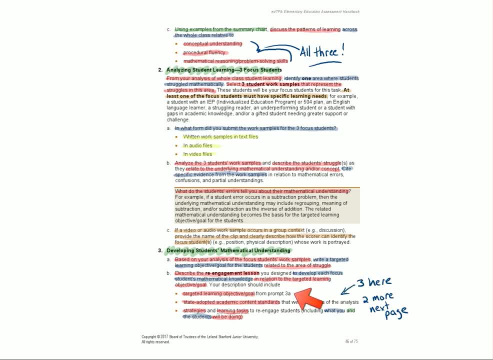 Your targeted learning objective, a goal somewhere in in your description of your lesson plan. Next, you need to set out the state adopted content standards that fit with this objective or goal. The third bullet point is the is the part you're probably most familiar with. this is actually what you're doing. 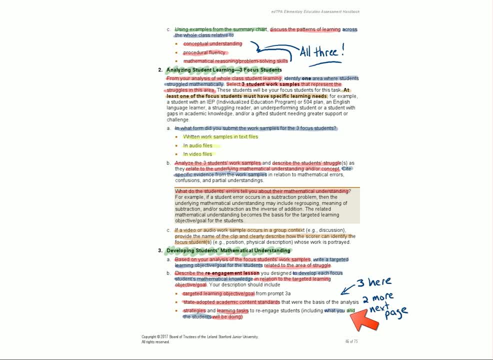 So what strategies and learning tasks are going to be happening in this lesson? Now? the essential piece right here is: you need to include in this lesson plan portion, include in your strategies and learning tasks what you were doing and What the students will be doing. this shouldn't just be about you, what you're doing. I will do this, then I will do this. 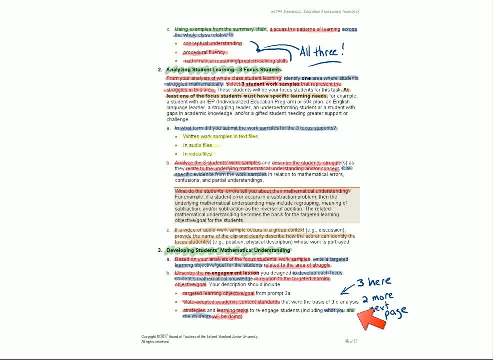 I will follow with this. you need to be including Students involvement as well, and you want students to be actively engaged, right? So they're doing something with the mathematics rather than just completing a worksheet. What are they doing in that task? So, if they're working with materials, what are they doing mathematically with those materials? 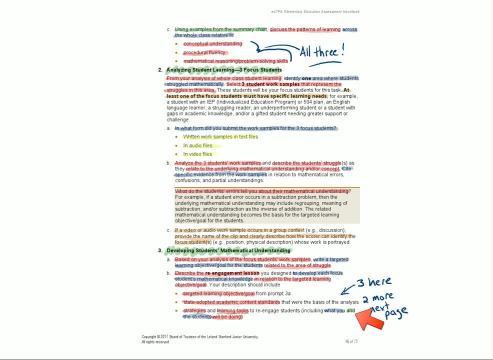 Keep all those good lesson planning ideas and mathematical and keep the mathematical focus in your planning. Alright, so I'm gonna go over the key points from this page. All right, so going back up to two, analyzing student learning, the three focus students, remember you want to. 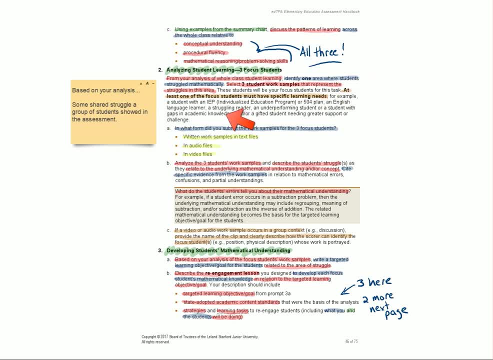 Focus on ones that have shared a particular struggle. based on your analysis, Some shared struggle a group of students showed in the assessment. So your three focus students shared something in common, a particular struggle. Next, as You write up your analysis of each of the three focus students, 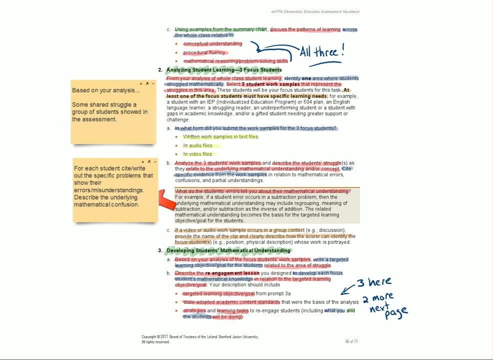 You want to write about the specific problems, that show their errors, misunderstandings and Describe the underlying mathematical confusion. Okay, so, for each one of the students. So you're analyzing the three students work samples and you're describing their struggles and, as I've said already, 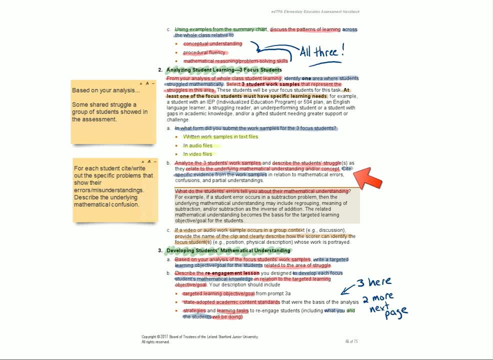 I'll say it again because it's very important. those struggles need to be supported. your, your definition of those struggles Needs to be just supported with evidence from their work, samples, from the actual problems, as you can see in problem 2a And you describe the problem the students struggled with all right. so particular evidence from the work samples. 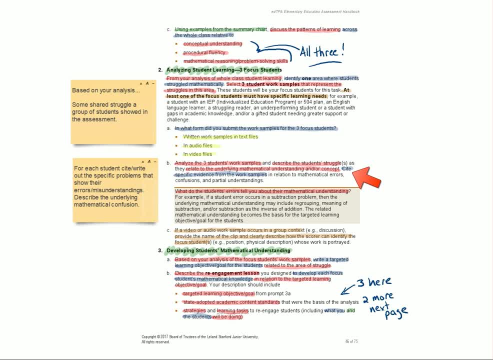 so that's very important. and lastly, from this page, They're going to be five parts to your lesson plan. We have the three of those five parts down here. You need to have the targeted learning approach Objective either the content standards. You need to have the strategies on learning tasks. that would follow, and on the next page We'll talk about the next two. 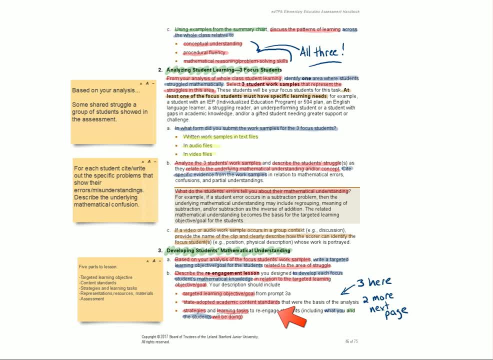 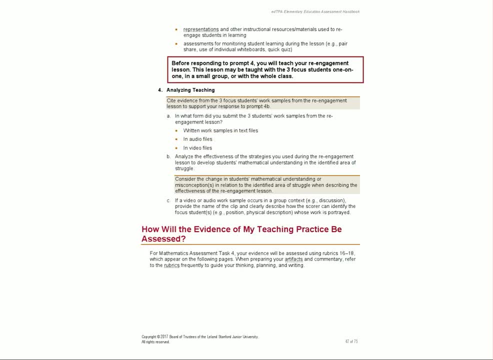 Representations, resources, materials and the last part being the assessment for the re-engagement lesson. So let's take a look at that. Okay, so the last two parts of the re-engagement lesson, you want to describe the Presentations and other instructional resource of materials that you're using. so this could be. 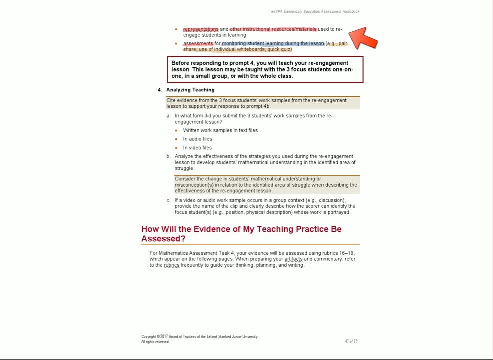 you know, whatever manipulatives you're using or whatever kind of worksheet you're using, or Any other kinds of tools like whiteboards or chart paper, those kinds of things that students might use to represent their learning. So keep that in mind. and the last piece of this is: 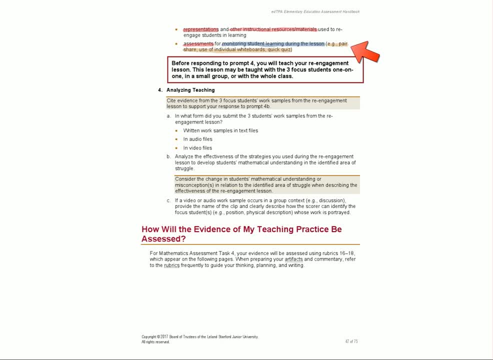 The assessments that you're going to be using during your re-engagement lesson. Now there's a key piece here. It's not an assessment That's just at the end of your Re-engagement lesson. it says for monitoring student learning during the lesson. So what you want to do in your lesson planning is set out certain points where you're checking for understanding. 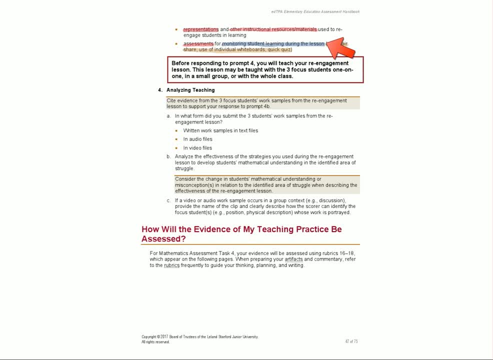 And this may be a question that's put out there. It could be some kind of gauge for understanding thumbs up, thumbs down. It could be some kind of short response quiz or something in there, Something simple, and you can see the examples they set out here. 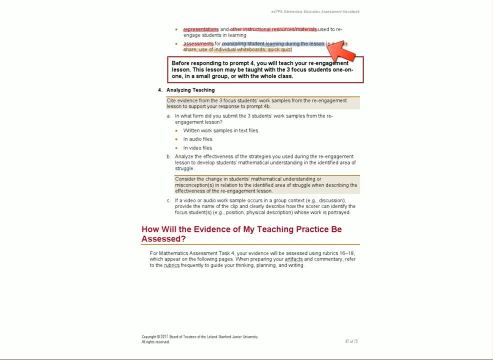 So this is monitoring student learning during the lesson. not just this at the end of the lesson, but during the lesson You're asking the kids to pair-share and you're listening in on how, what they say to one another, or you're having them report back. 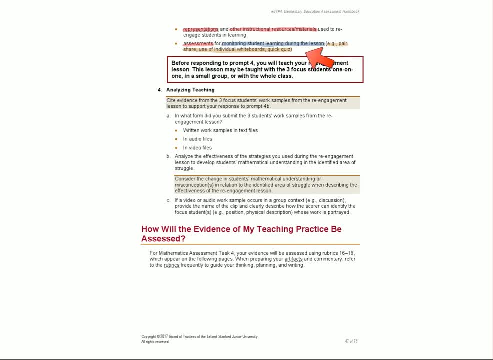 what their partners said. the kids might use whiteboards and Show you what they're thinking and turn them around and you can see all the kids whiteboards at once, or you could be walking around the room looking at what they're doing On their whiteboards- a quick quiz along the way. so this is really, really important because you're going to need this. 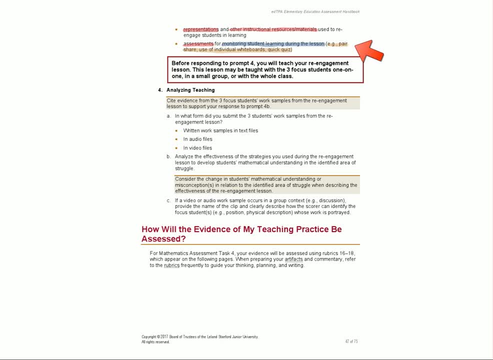 for your Write-up on the effectiveness of the lesson. so let's go over This part real quick before we go on. five parts to the lesson plan. Again, you want to have a targeted learning objective. you want to set up the content standards, You want to set out the strategies and learning tasks You'll be using and, from this page, the representations resources. 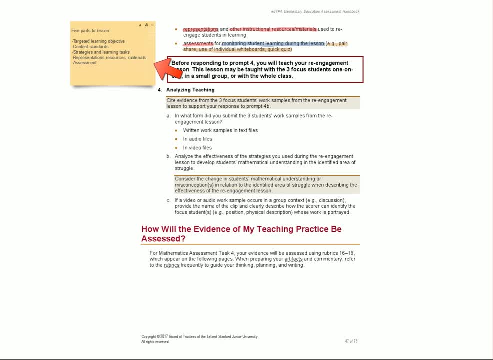 materials that will be involved. and then, finally, the assessment to monitor student learning during the lesson. okay, to monitor student learning during the lesson. what are the multiple ways that you'll be checking for understanding along the way? next, you have to do this next part before you write up the next. 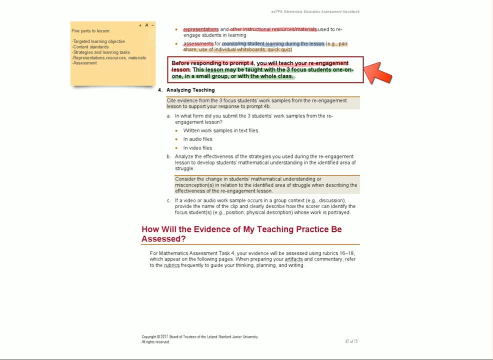 section of the commentary other. you actually can't do it without doing this first, so you need to actually reteach the lesson. so, before responding to prompt four, you want to reteach the re-engagement lesson, and this lesson may be taught with the three focus students- one-on-one and small group- or with the 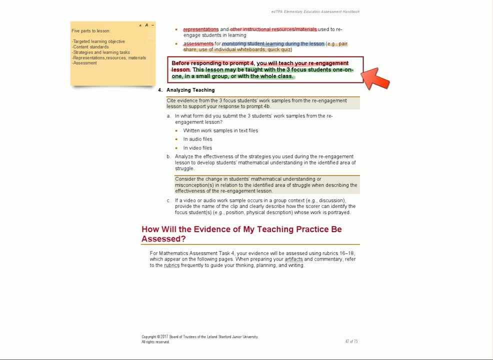 whole class all right. so just make sure that you're doing all of these good things along the way. but here's something to anticipate before you teach, as before you teach the re-engagement lesson. your re-engagement lesson is about changing the students mathematical understanding in relation in the area that they struggled in. so you want to be thinking. 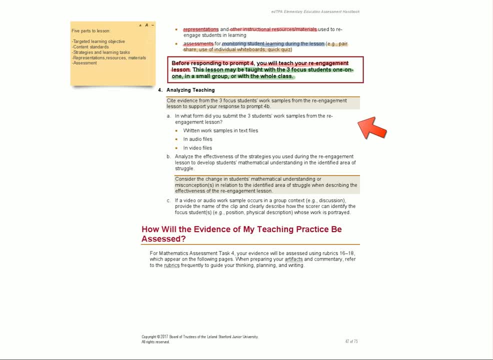 about that. as you're teaching, as you're teaching your students, how is this lesson? ask yourself, how is your teaching? how is this lesson? how are the students engaged in a way that's changing their understanding in that area of struggle? that's the most important part of the re-engagement lesson: the re-engagement. 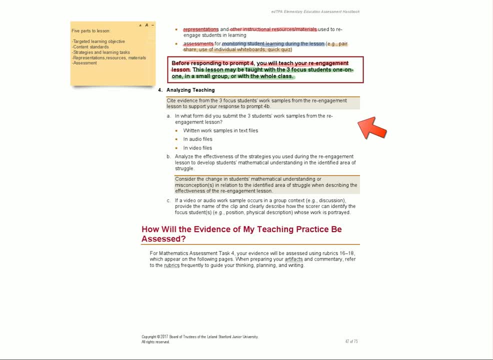 lesson is meant to change understanding in relation to the area of struggle, so let's go ahead and go down to the analyzing teaching section now. alright, so you've taught the lesson and then the evidence you've collected from the three students, work samples. so whatever work you've had them do in the 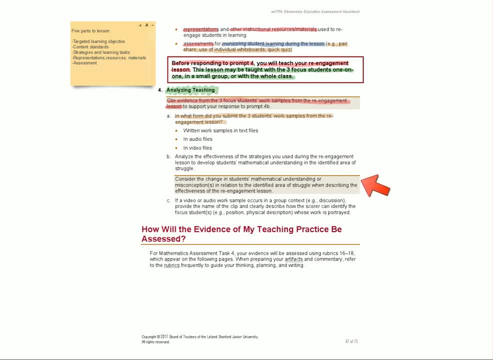 re-engagement lesson. you're gonna respond to these prompts, alright. so the first one is a simple question again: in what form did you submit the three students work samples, the re-engagement lesson, and you have choices: work samples, audio files or video files. now you could imagine- and this might be a smart way to think about it- 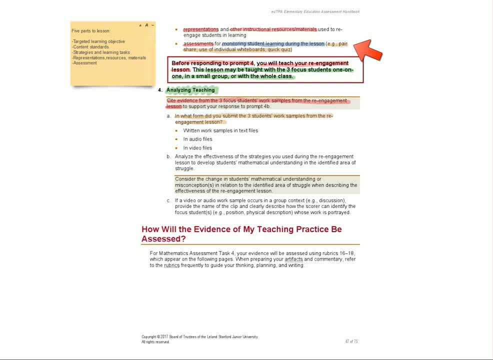 if you're doing some kind of ongoing assessment or monitoring student learning throughout the lesson, then a video would be very supportive of that kind of would allow you to collect evidence of that very readily. you wouldn't have. you would have more than one artifact you could talk about, write about what particular students are. 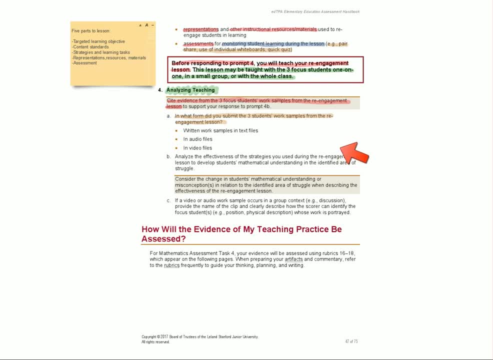 doing at different points in time within the video. all right, so you need to keep these in mind. all right, because you're looking for change in students understanding b, you want to analyze the effectiveness of the strategy you used during the re-engagement lesson to develop mathematical understanding in the 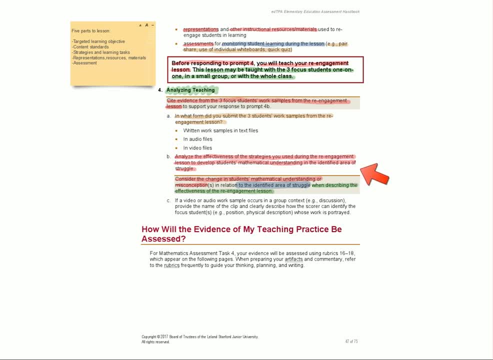 identified area of struggle. okay, so what? based on what you see in the video or in students work, what's changed for your students? all right, and it's best described here. consider the change in students mathematical understanding or misconceptions in relation to the identified area of struggle. 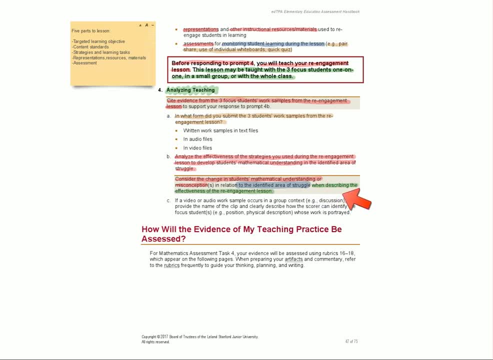 when describing the effectiveness of the re-engagement lesson, all right. so your analysis has to be about changes in thinking, changes in mathematical thinking for your three focus students, all right. and then c, and this goes for all video: if you're focusing, if you want to describe what, 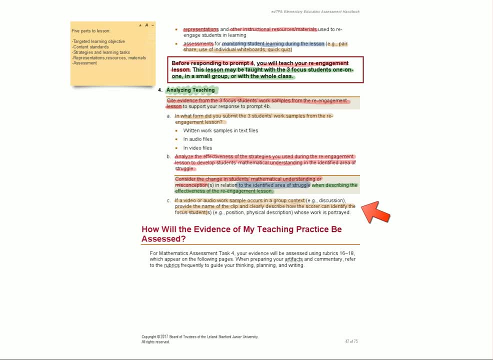 any particular student's doing and it's not clear which student is which you need to give some identifying mark to say this particular student was wearing the red sweatshirt or something like that. all right, so some points for this particular page. first off, we've talked about the five points to the lesson. okay, make sure you've hit all. 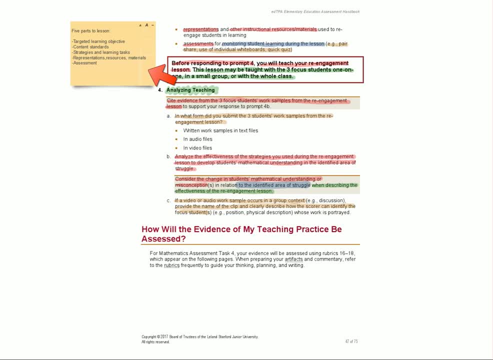 five of these points and don't do it just because it's an ed tpa requirement. if you do these five well, then your re-engagement lesson, your actual teaching, will be more successful. so really, really give good time to this so that you will have a good lesson, lesson to teach your students. 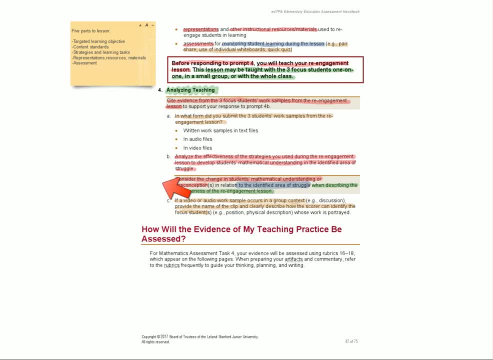 okay, and the important part down here, when you're thinking about the effectiveness of the lesson, describe the effectiveness of your engagement lesson in terms of change in students mathematical understanding. okay, so it's that. it's how they think differently now because you've taught them that matters in your re-engagement lesson. 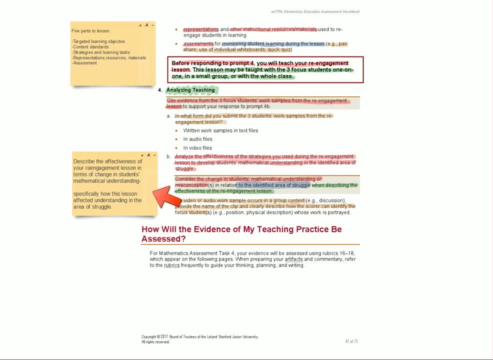 that's what an elective, effective lesson should do, um, and then, of course, whatever change that is that you're describing should be focused on that area of struggle that you identified earlier on in your analysis. all right, so let's go on to the rubrics for this task. they're just three. 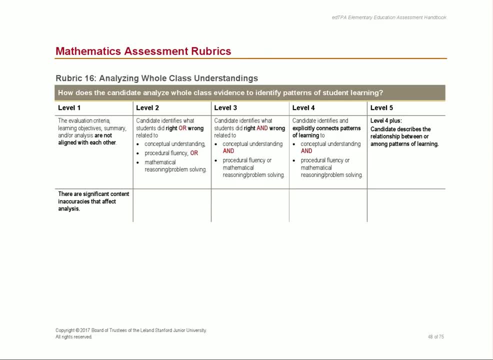 for the mathematics task and the first rubric for the mathematics assessment task is analyzing whole class understandings. all right, and you can see with level three this is a passing level. the candidate identifies what candidates did what, i'm sorry. the candidate identifies what students did right and wrong related to conceptual understanding and 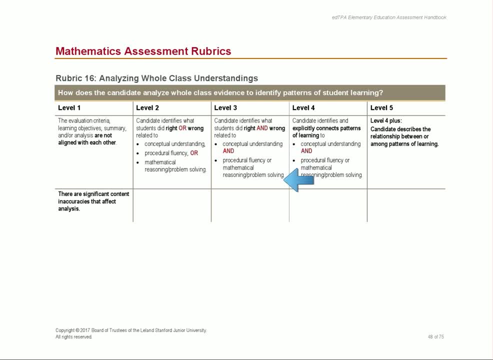 then you get a choice: procedural fluency or mathematical reasoning or problem solving. so you really have to do two of these. but you must do conceptual understanding for a three okay. so it's a base requirement, but you really should be shooting for a four, because that will encourage you to do really good. 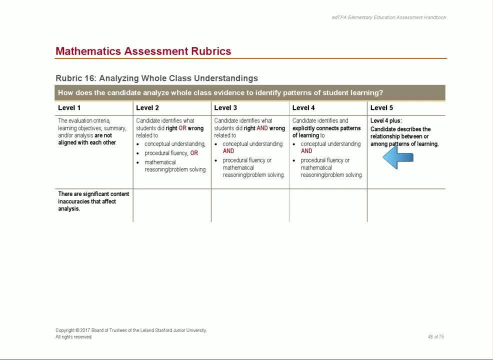 mathematics teaching. so let's see what four says. under level four, the candidate identifies what's and explicitly connects patterns of learning. so you can see the change already. the candidate identifies what students did right and wrong, versus a focus on patterns of learning. okay, so this is looking across class in ways and across the mathematics, instead of just a binary. 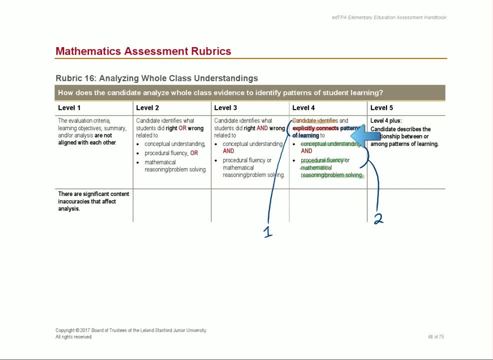 two-dimensional right and wrong focus. now you can see that the next part is similar. you have to have a focus on conceptual understanding, but you want to be able to talk about procedural fluency or mathematical reasoning and problem solving. okay, so the difference between a three and four is essentially a difference between right and wrong and patterns. 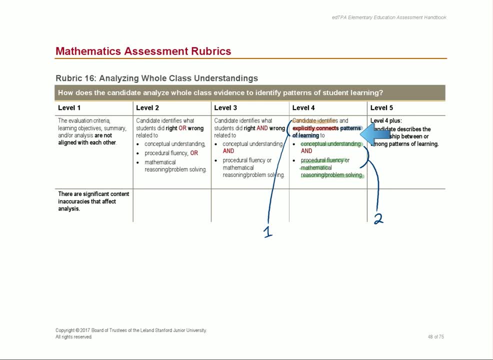 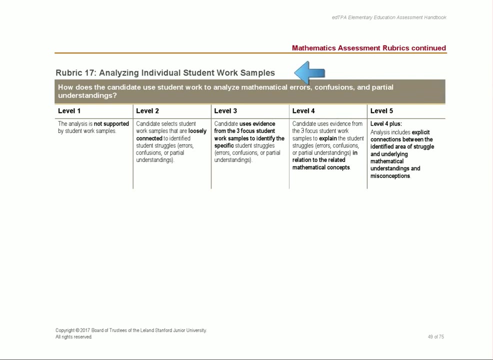 of learning. so you have a focus on patterns of learning. you'll move to a four, so keep that in mind. the next rubric for this one analyzing individual student work samples. so these are your three focus students. how does the candidate use student work to analyze mathematical errors, confusions and partial 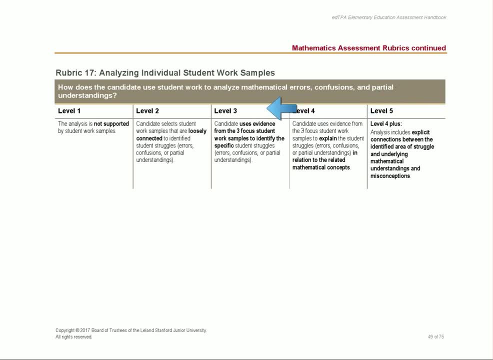 understandings. for three, which is passing, the candidate uses evidence from the three focus student work samples to identify the specific student struggles. okay, so you looked at your student's work and you found where they're struggling. that's a three, a four and we want to take our work to the four. 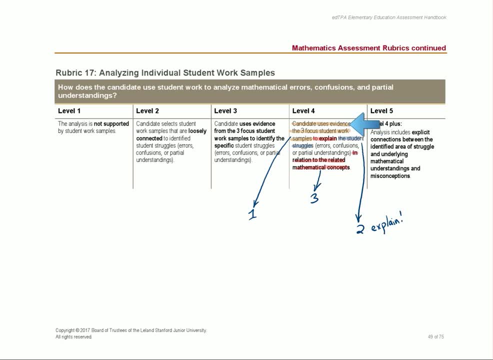 in a four, the candidate uses evidence from the three focus student work samples. so far the same and here's a difference. to explain: the students struggles, okay, and the other addition here is in relation to the related mathematics. the student struggles and the other addition here is in relation to the related mathematics. 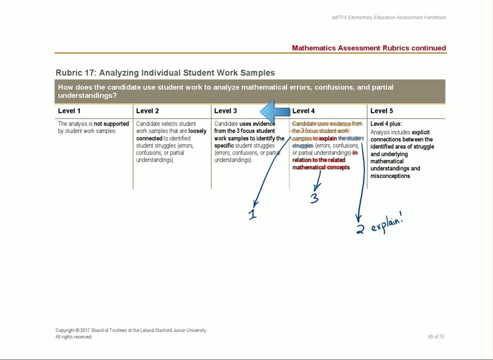 concepts. So the difference between a 3 and a 4 here is that in a 3 you're just identifying struggles. in a 4 you're explaining the struggles in relation to the related mathematical concepts. So giving detail about the struggles, explaining what's going on with students work, will move you from a 3 to a 4.. And 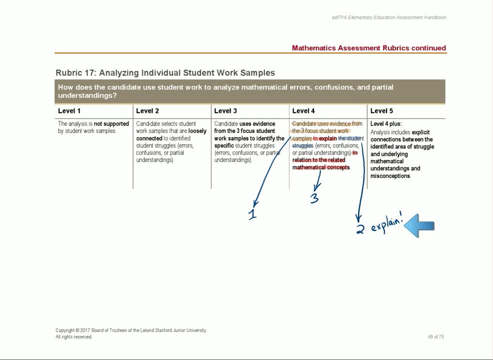 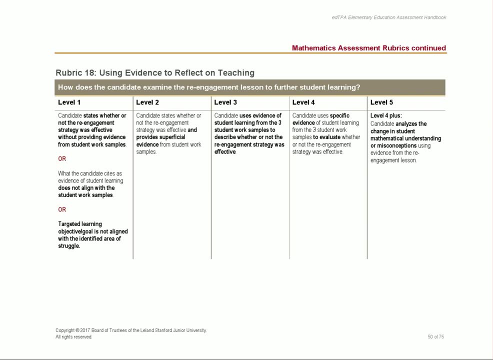 of course this is the key word for this particular rubric. explain The last rubric 18, using evidence to reflect on teaching. How does the candidate examine the re-engagement lesson to further student learning For a 3,, which is: 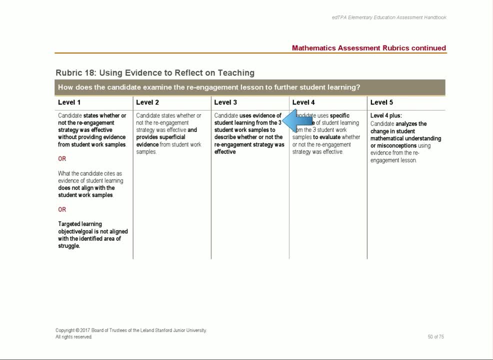 passing candidate uses evidence of student learning from the three student work samples to describe whether or not re-engagement lesson was effective. Okay, So using evidence to say whether it was effective or not, Let's see what 4 asks for, And we do want to shoot for 4's. There's a 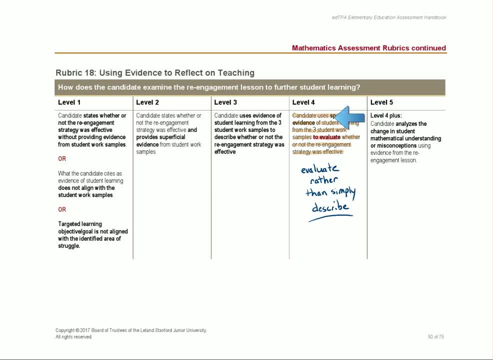 key word in this, one that's different than the other. So, if we look here, candidate uses evidence of student learning, candidate uses specific evidence. Okay, So that means you're looking at particular things the students are doing that are related to the focused mathematical. 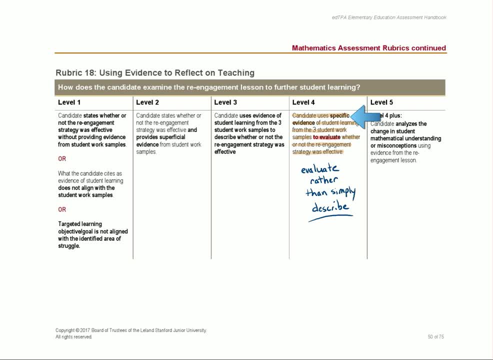 data And we're looking at what we're looking at right now And what we're looking at from two different variables. content: the targeted learning objectives. So the candidate uses specific evidence of student learning from the three student work samples to evaluate whether or not the re-engagement strategy was effective. 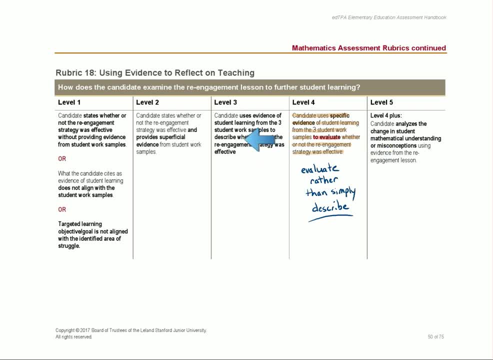 So a difference here is for a 3 to describe whether or not the re-engagement strategy was effective and a 4 is to evaluate whether or not the re-engagement strategy was effective. To evaluate would mean that you have some kind of criteria, some kinds of. 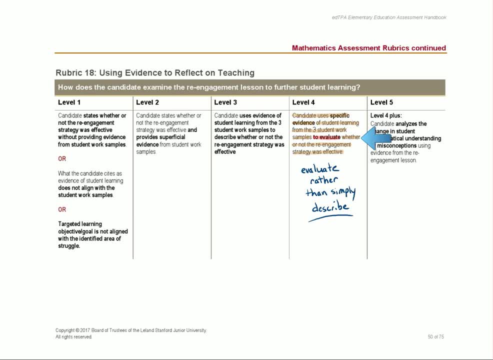 things you were hoping that should happen in that lesson. So if you're going to evaluate the effectiveness of your re-engagement lesson, base your evaluation on the criteria you set out in your targeted learning objectives. If you look at your targeted learning objectives for that, 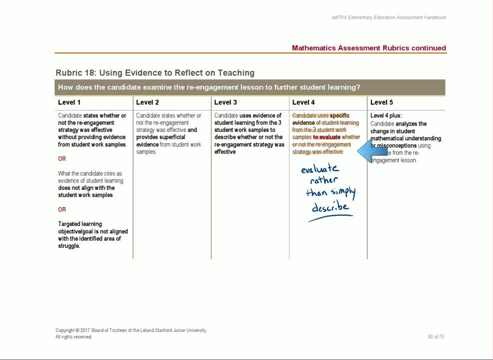 re-engagement lesson and students show good evidence that they meet those things, meet those objectives, or they might still struggle in regards to those objectives, then you're evaluating the effectiveness of the lesson, Not just saying students seem to be pleased with their work and they have. 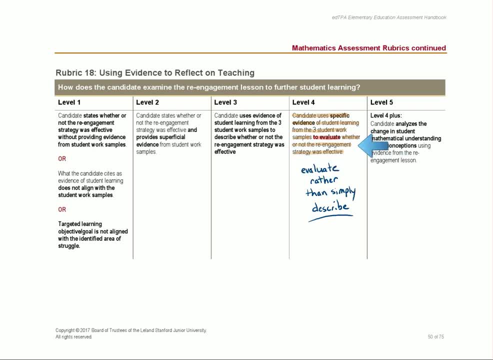 good answers. You want to evaluate your work in your re-engagement lesson relative to the criteria you set out in your lesson planning. So the big idea here is evaluate rather than simply describe, And that will move you to a 4.. Task 4 is a long task.